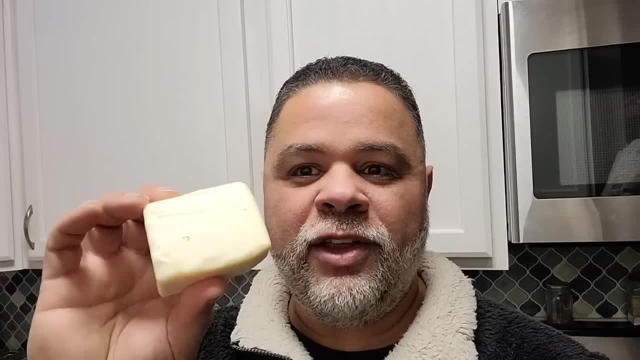 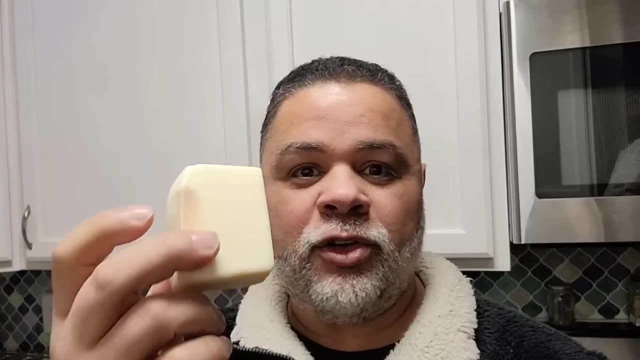 soap like this will be very barterable. Now, this here is the very first bar of soap that I've ever made, Believe it or not, it's over seven years old, going on eight years, and it's still good. It still works. I have many more. I made a batch about eight years ago just to try it. 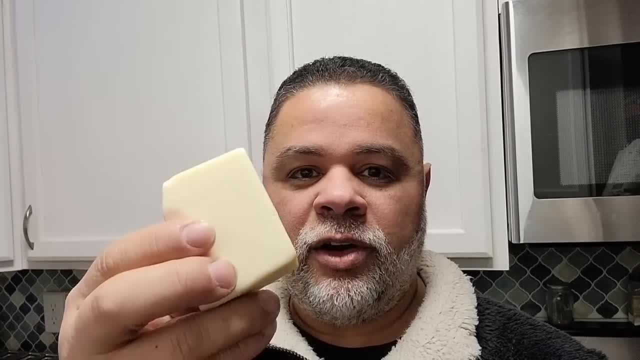 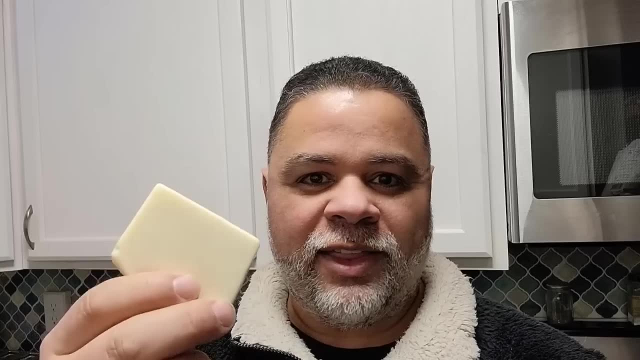 and it still works. And this is a very simple soap recipe. It has water, it has lye and it has oil and that's it. It doesn't even have any oils to make it smell good or anything like that in it, It's just a. 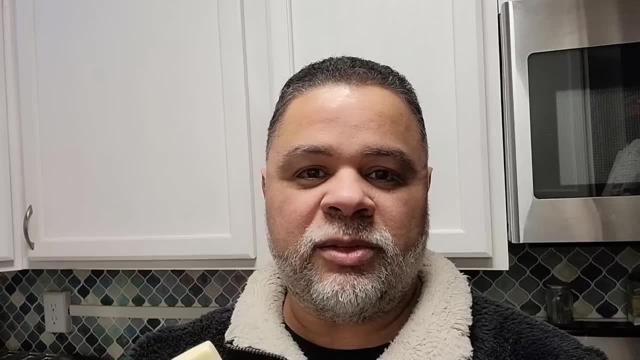 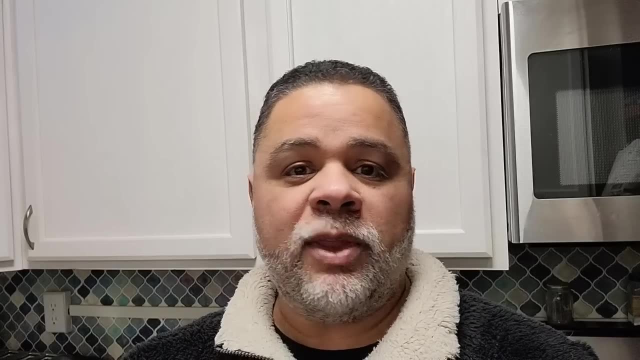 basic soap recipe And I believe that if you learn how to use this recipe and make it and have the things that you need in order to be able to make soap in the future, that you'll be a lot better off than most people. Because ask yourself something, ladies and gentlemen: how many people 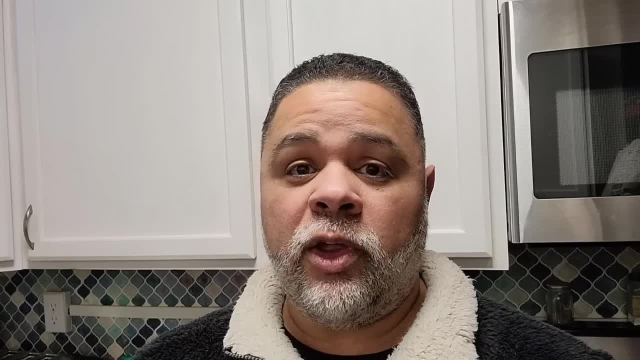 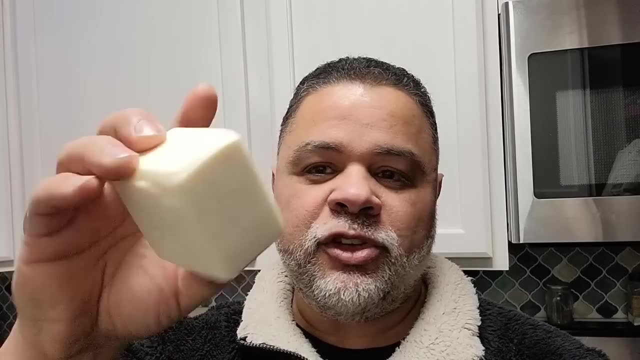 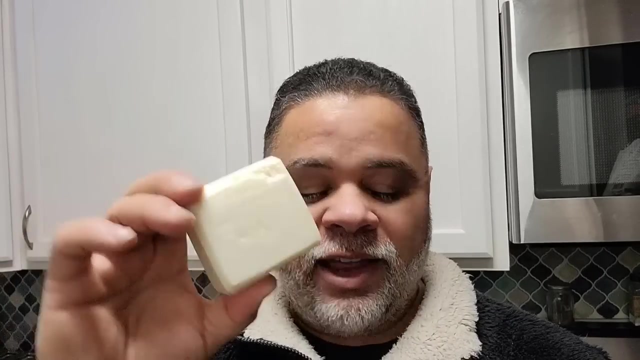 that you know can make their own soap. Well, those are the people that are going to be able to barter this with. Now, this is just a basic soap. I also made another one that's pretty basic. that's just with a little bit of peppermint essential oils in it, And it smells pretty good, All right. 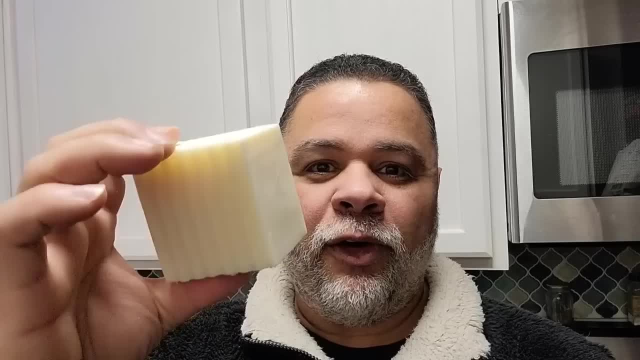 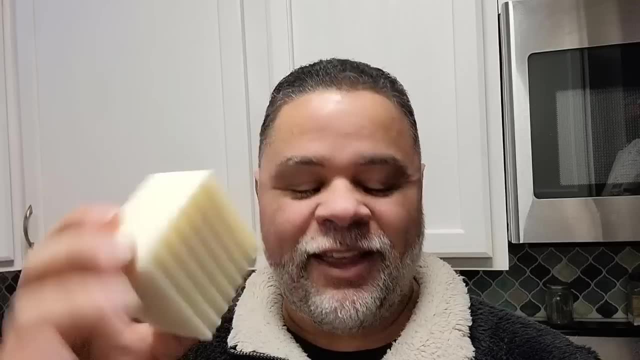 doesn't have a lot. And then I made another one that's a little bit more in depth, that has peppermint and it also has some botanical smells in it, ladies and gentlemen. So it smells very nice. So you can take this soap recipe that I'm going to share with you, and you can pretty much. 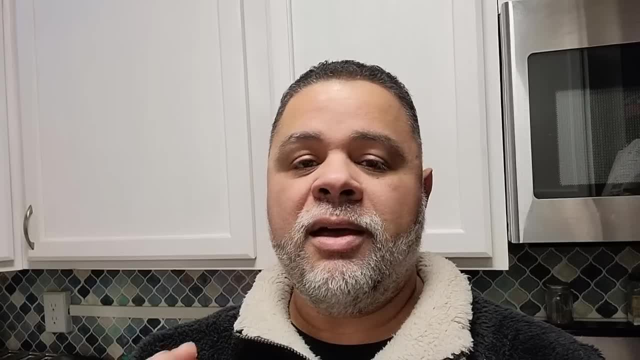 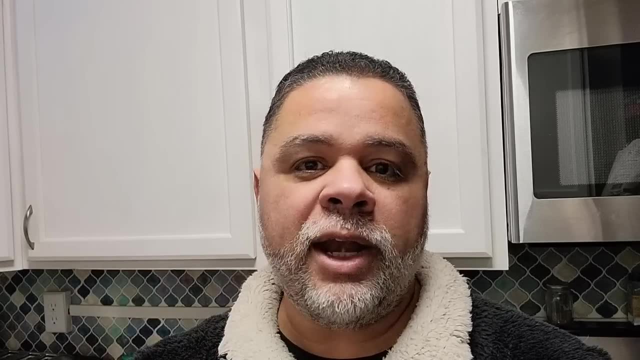 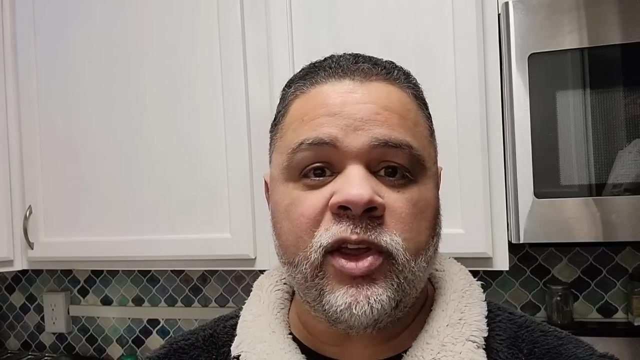 add anything to it that you want. Now let me cover this real quick. I'm sure that there's a lot of gurus. All I'm trying to do here, ladies and gentlemen, is show you how to make a basic soap. Today, what we're going to do is we're going to make our basic soap recipe. That way you can see. 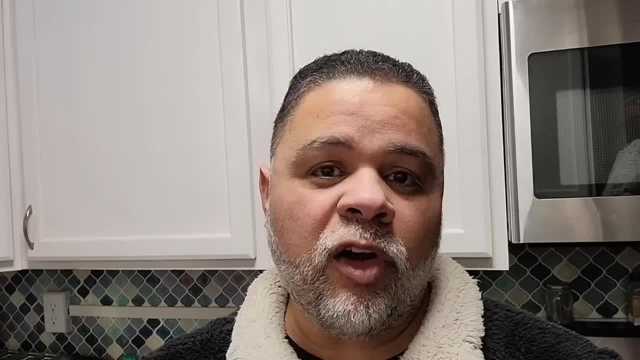 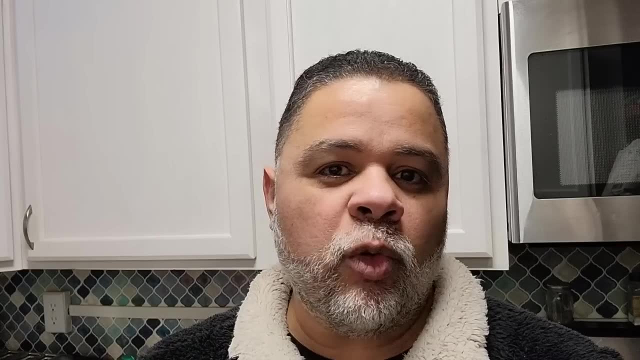 how easy it is, And then we're going to add some vanilla beans to it, along with some black earl tea, I believe it is. We're going to grind that up and add it towards the end, And then we'll show you what it looks like once it's hardened and it's come out of the mold. All right, so let's get. 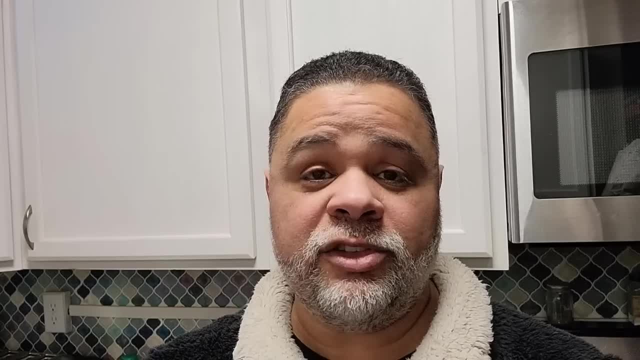 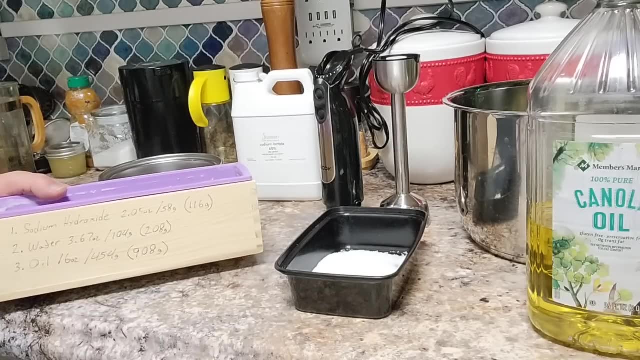 started. Let me show you first what we're going to need in order to make this Very easy, ladies and gentlemen, So don't be afraid or intimidated of doing this. So here, ladies and gentlemen, is everything that we need in order to make our soap. The first thing, 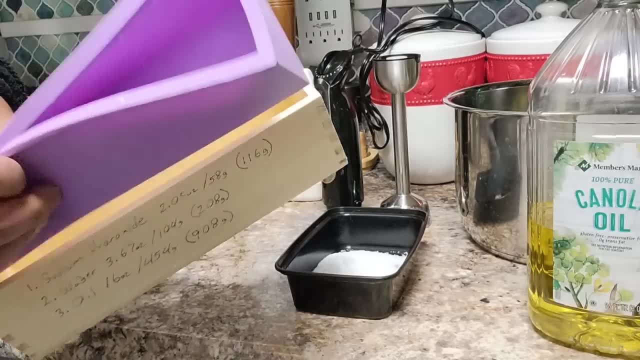 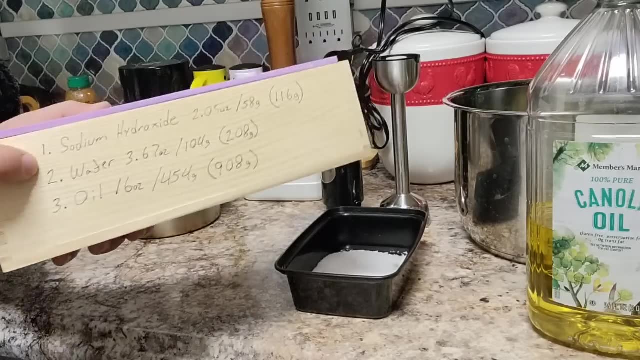 is we're going to need some kind of a mold. You can make your own if you want. I purchased this one a while back, Easy to use. As you can see, I've already used it before. But here I went ahead and wrote down my recipe, And the recipe is sodium hydroxide or lye. Many people know it as 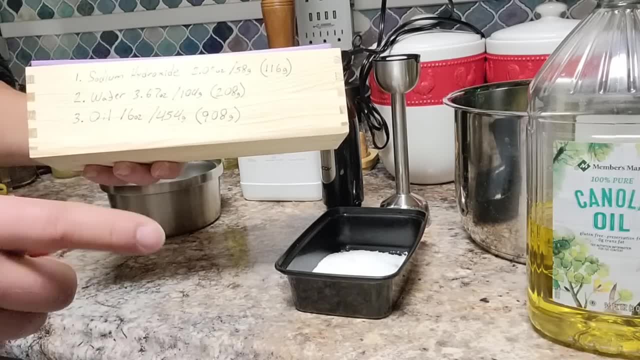 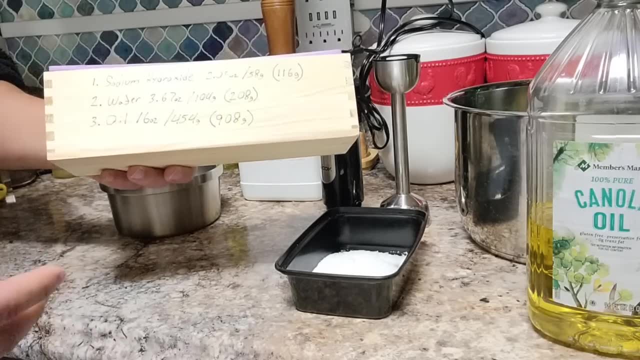 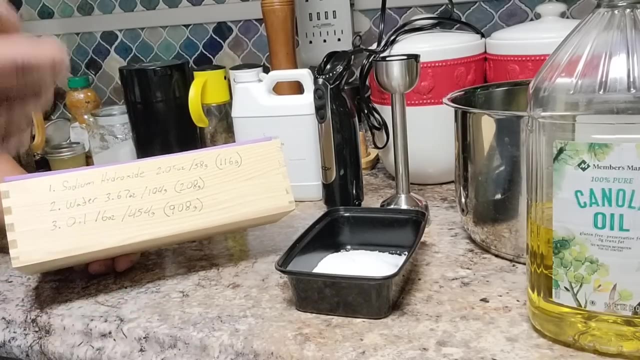 lye. We're going to need water, preferably distilled, but I've always used reverse osmosis, just fine. We're going to need oil. In my opinion, any kind of oil would do. Now, I do understand. like I said before, there are some soap gurus out there that are going to say, well, if you use so, 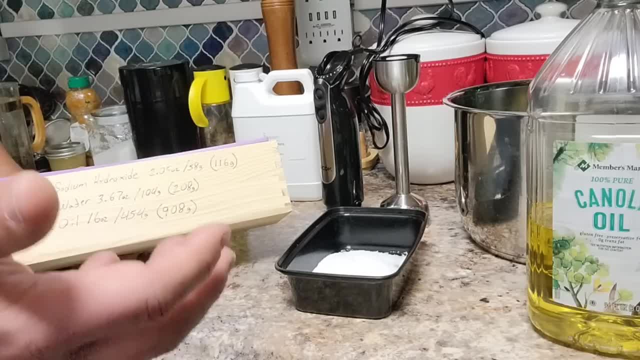 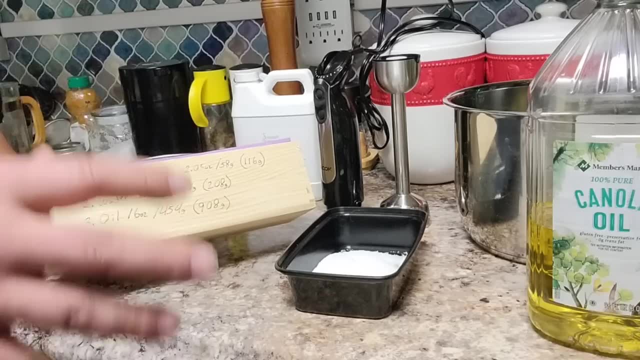 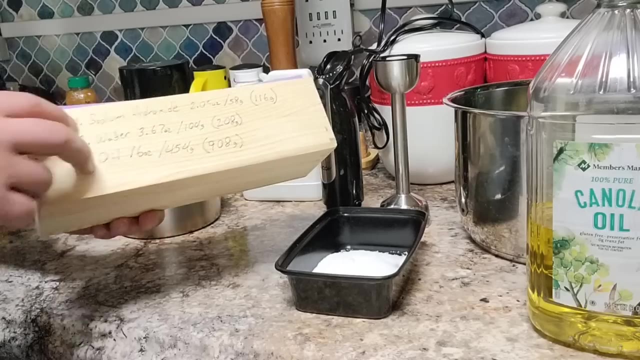 much of this oil and make him out dry. if you use so much of this oil, your super fat has to be this level or things like that. But my goal here is to encourage you to make a basic bar of soap. That way, you know how to do it, should you ever have to. This is pretty much all of the ingredients that 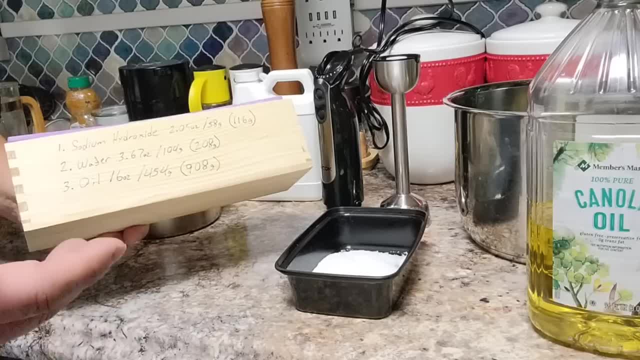 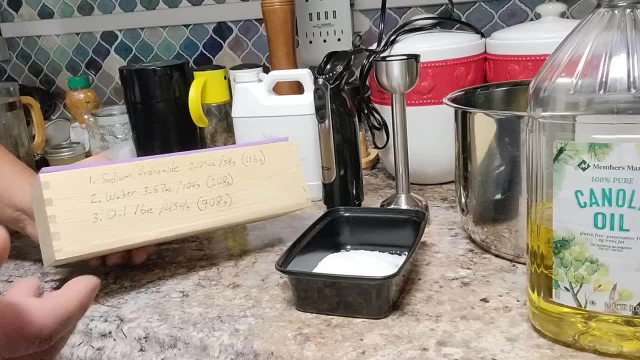 you need Now. you can add essential oils to it to make it smell better. You can add things like what we're going to add today, which is some vanilla beans and some tea to it as well, so that you can have some kind of an exfoliating effect from the soap and give it that smell. This is something that you 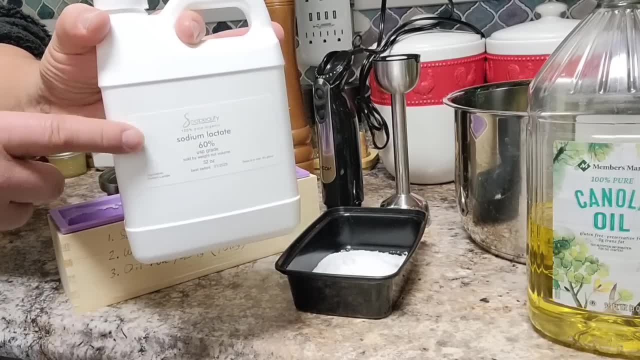 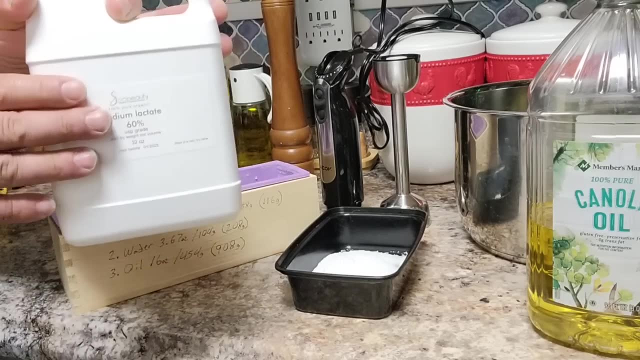 can also use. This is sodium lactate And you only need to use a little bit of this, but you don't have to use this. This just helps the soap harden a little bit faster and a little bit harder. I use just a tiny bit like maybe a 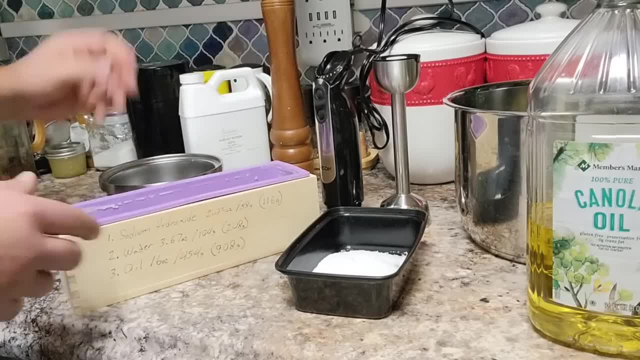 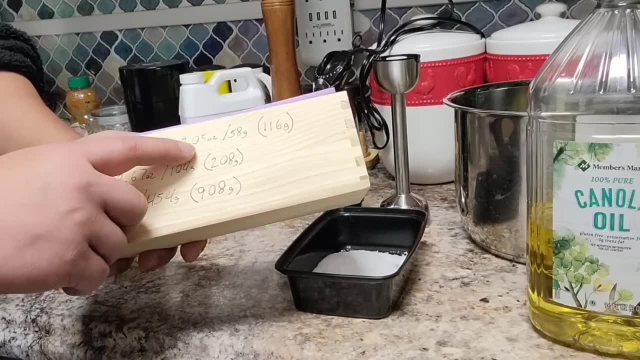 half of a teaspoon for an entire batch. Now, something that I didn't cover is this recipe right here, As you can see, the sodium or the lye, it's asking for 2.05 ounces or 58 grams for one batch, But this 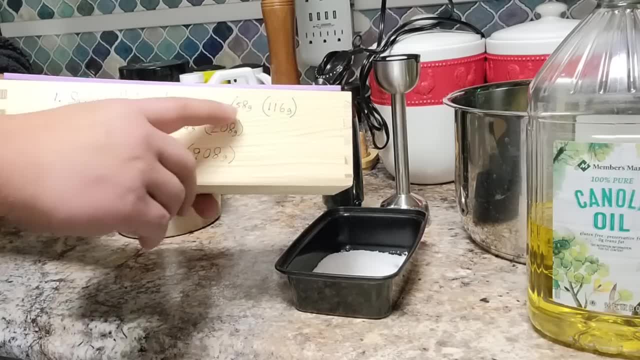 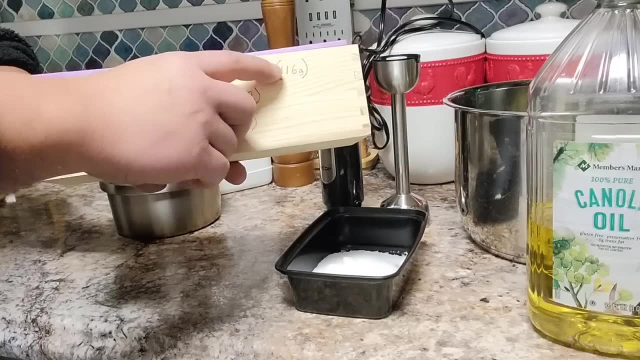 right here this container. it takes 116 grams. It takes a double batch, So I went ahead and wrote down the ingredients that we need for one batch and a double batch as well, because a double batch will fill this entire mold right up. 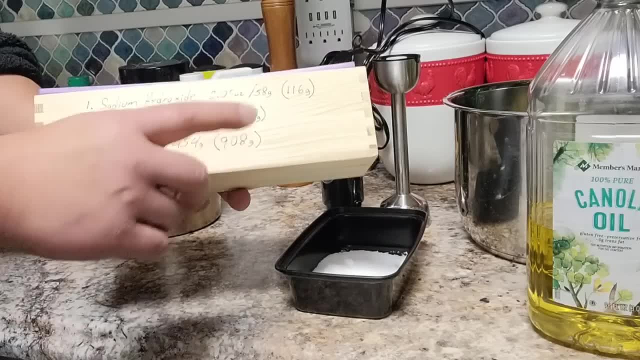 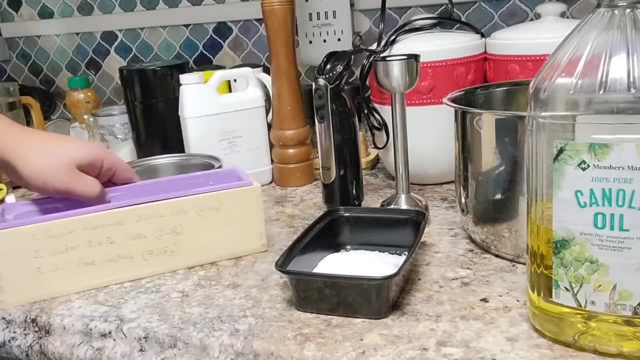 Same thing with our water, same thing with our oil. So it takes 208 grams of water, 908 grams of oil. Of course, here's our lye, And with the lye you have to be very careful. ladies and gentlemen, Do your. 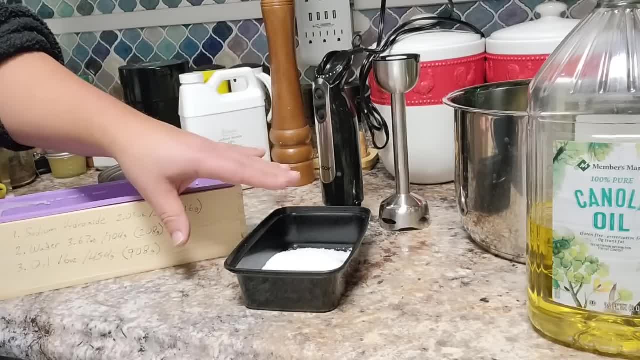 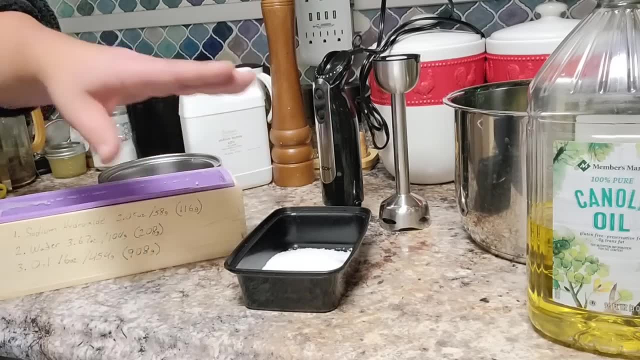 research. This can really hurt you if it gets on your skin or your eyes, So make sure that when you handle this, you have the proper PPE. When I actually put this into our water, we're going to go ahead and do it outside, because it does release gases. 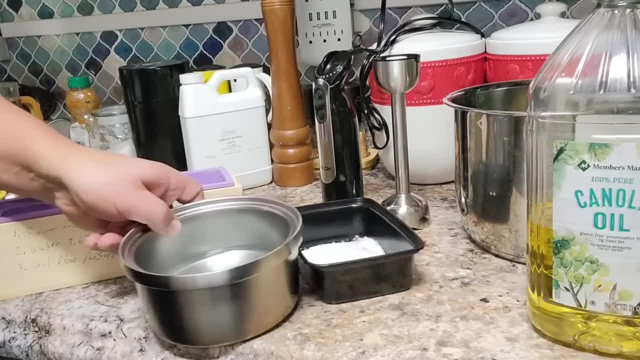 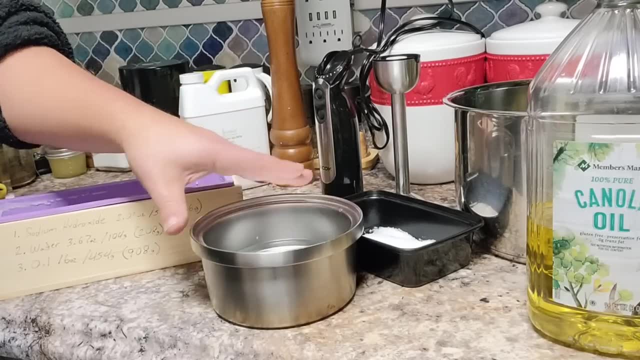 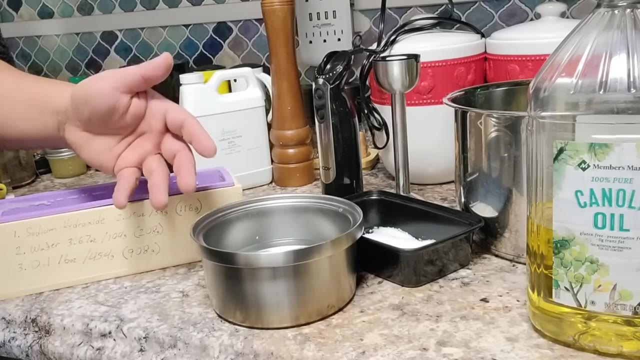 It also gets very hot getting to the point where the container where I put my water. I already have my water pre-measured in this container. I always use a metal container because if you use a glass container, from personal experience this is that glass container can crack because this gets hot very, very quickly. 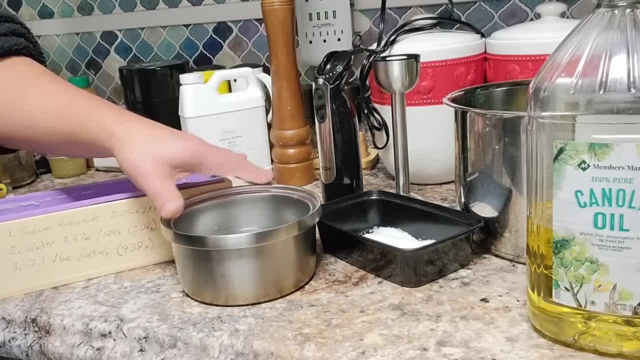 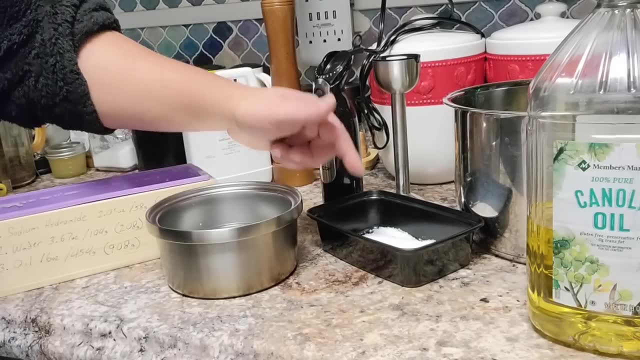 And one thing that I've always done, and one thing that I've heard recommended an awful lot, is that when you do add the water and the lye together, that you always add the lye and the oil together, And that's why I always add the lye to the water, never the water to the lye, Because, again, when you add these two, 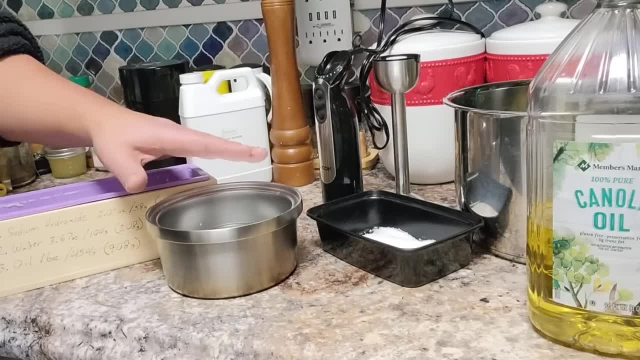 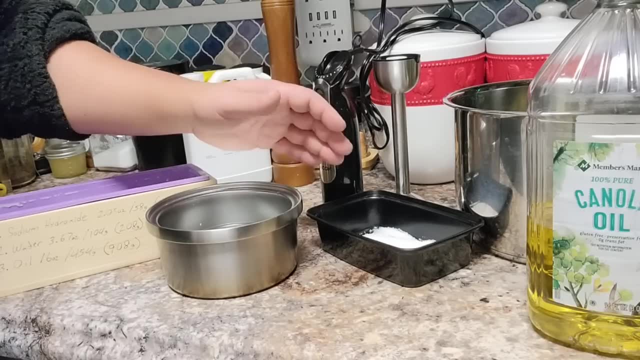 ingredients together. it's going to get very hot, probably about 180, 190 degrees, in a real quick hurry. So you don't want to add water to the lye and then have it produce that much heat without all of the water. 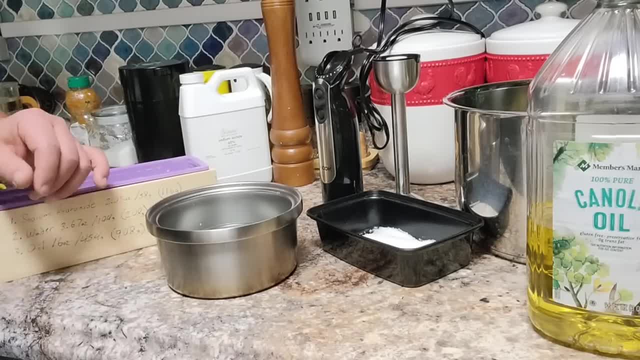 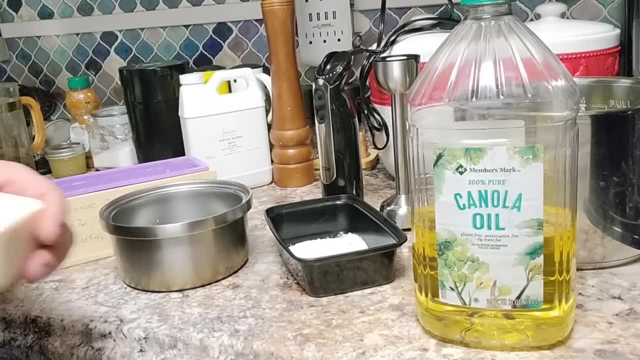 being added in there already. So, in other words, dilution is the solution. okay, Again, you can use any kind of oil that you want. Ladies and gentlemen, this soap right here. I ended up using some extra virgin olive oil, just extra virgin olive oil. 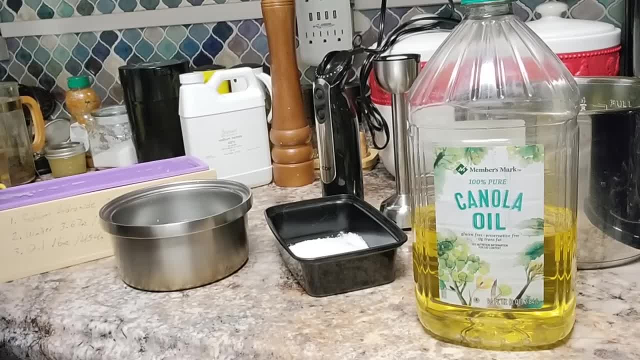 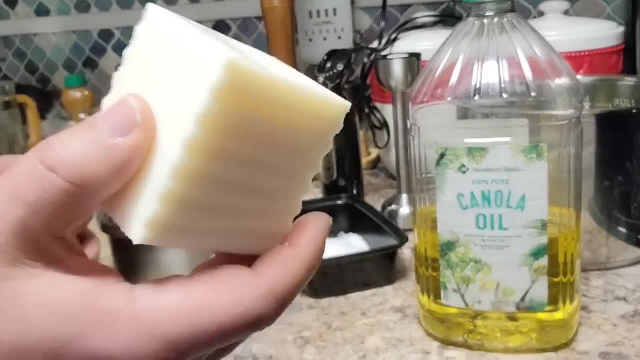 and that's it. Let's see where's the other bar. This soap right here. I used some extra virgin olive oil with some coconut oil, about a 60-40 split, You can see it came out just fine. And this soap right here. I think I remember. 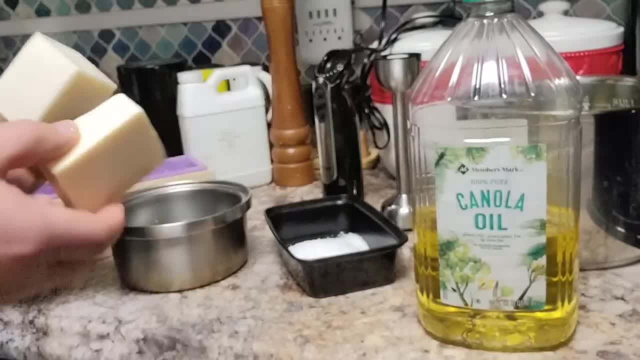 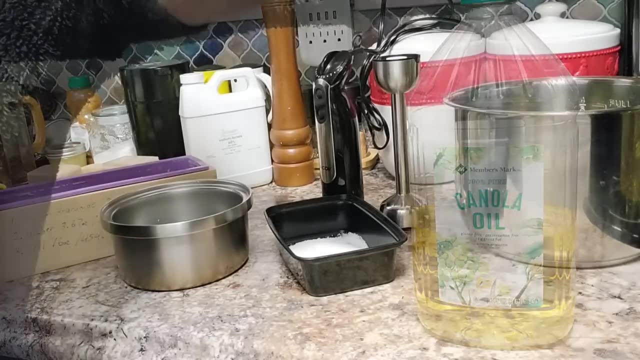 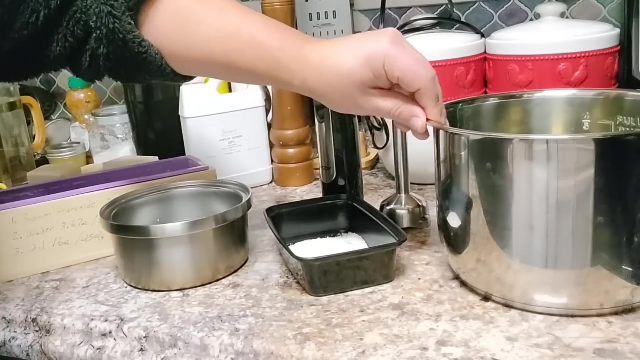 making this with corn oil several, several years ago. So any oil that I've ever used, it's always worked right And it's always done what soap is supposed to do, which is clean. So we're going to use canola oil, and I've already got it pre-measured: 908 grams of oil. So now what we're going to do is 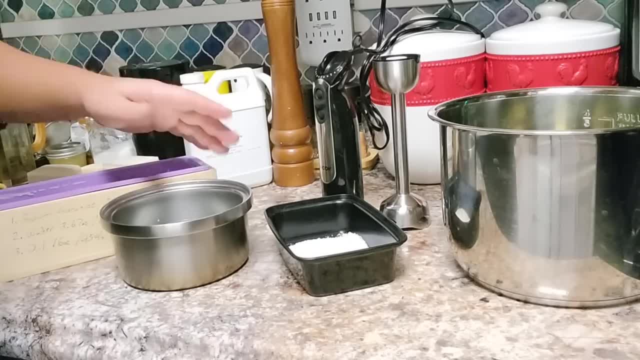 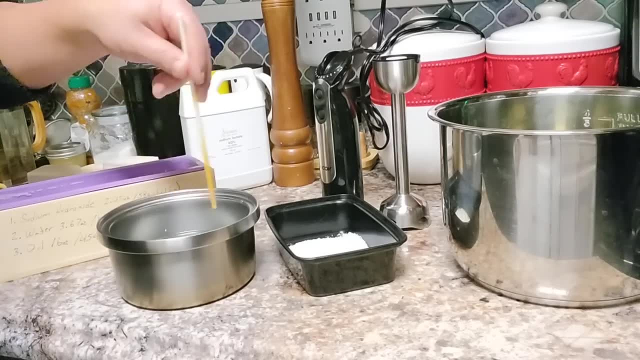 we're going to go outside. I'm actually not going to take you outside. I'm going to go outside. I'm going to mix this together, and I've got a handy-dandy chopstick here that I use in order to go ahead and mix it really well, And then I'll bring it back inside when there's no more vapor. 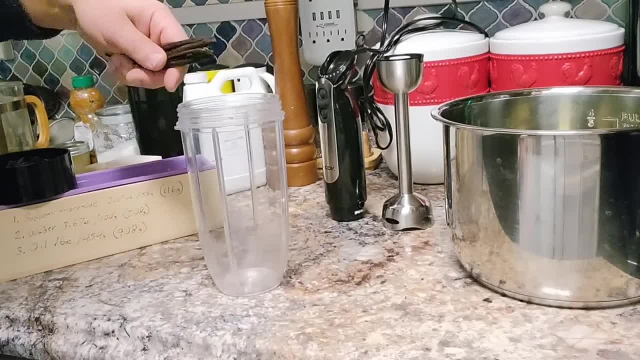 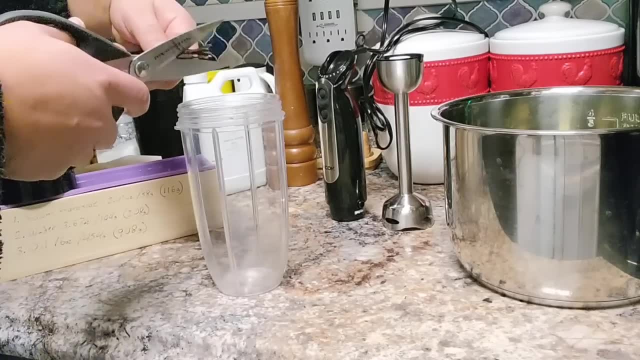 coming out of it. The water is outside, ladies and gentlemen, cooling down. We're going to go ahead and put. I got some beautiful vanilla here right, Nice natural vanilla, or Madagascar I believe it is, And this vanilla. 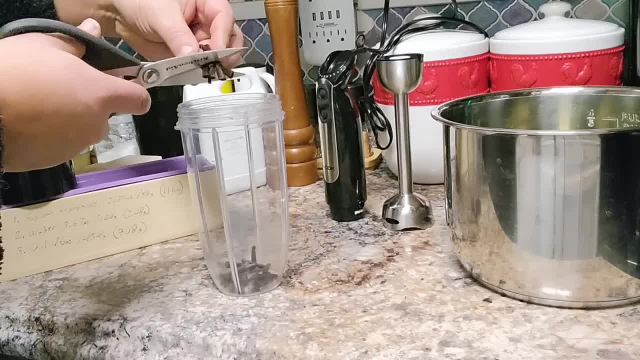 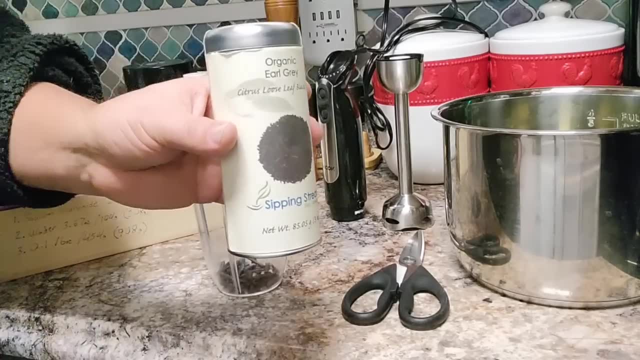 believe it or not, somebody- one of you all- sent this to me about a year and a half, maybe two years ago, and I still have some of it, So we're going to put that in there. This is really really good tea. 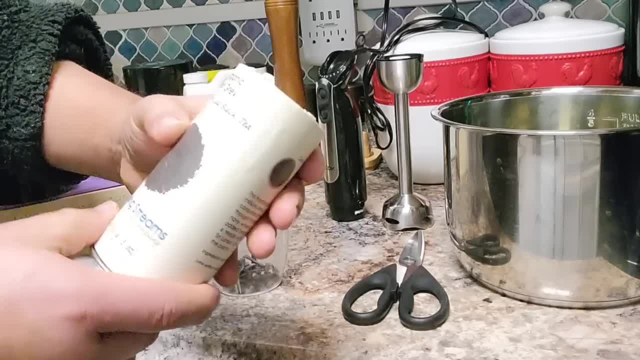 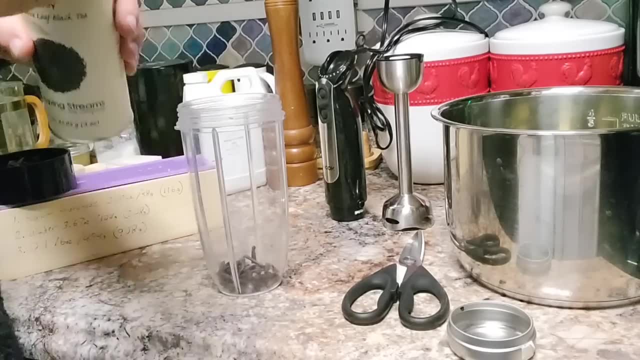 and it smells so good. That's why I decided to use this one. It's a what's it called Organic Earl Grey. I thought it was black, but oh my goodness, it smells really good. So we're just going to put a good. 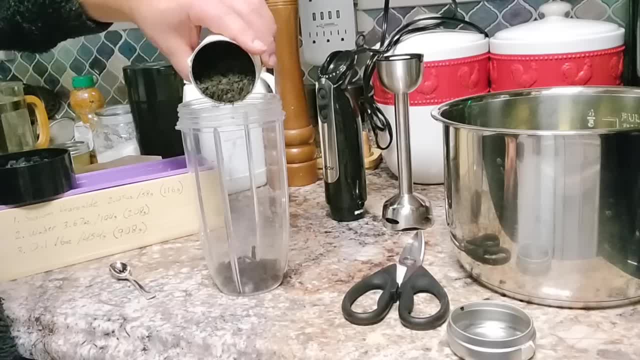 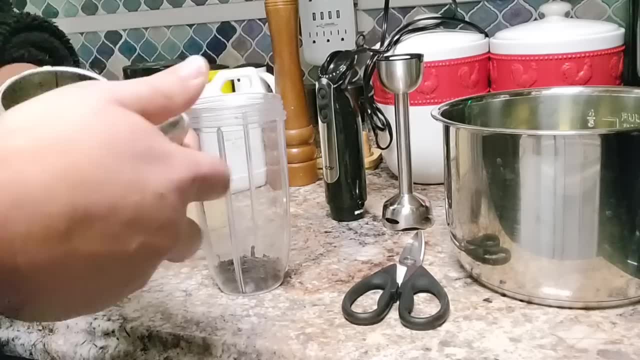 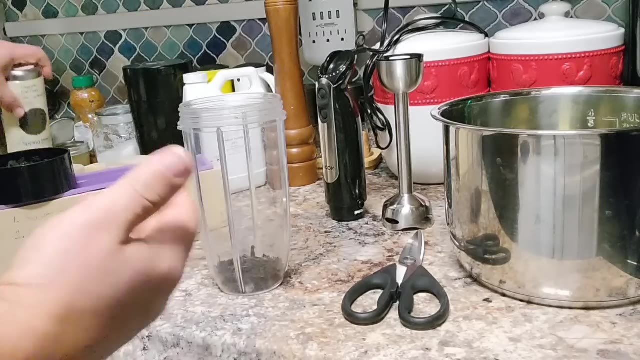 amount in there. I'm not going to be shy with this, because through past experience I've noticed that when you think that you're putting a lot of like, let's say, essential oils in there and you think it's going to smell really strong, it doesn't, even if you put a good amount, because it disperses. 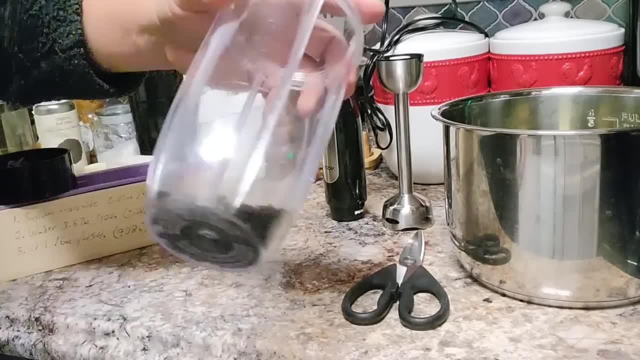 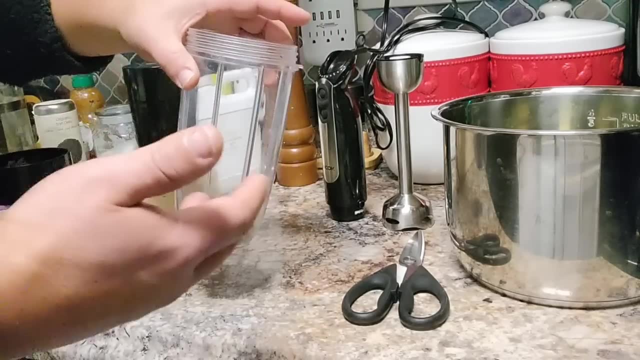 itself, or it homogenizes itself really well. So, as you can see, this is what we got right here. We're going to grind this up and then we're going to save it to the side for after we've pretty much gotten our soap done and it's achieved a trace right, So we'll be right back with that as well. 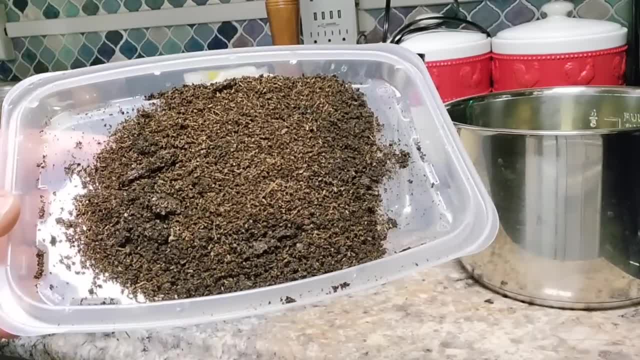 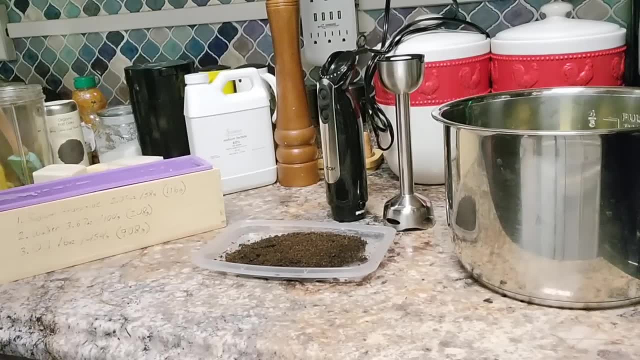 And that's what it looks like after we put it through the grinder or to the blender. I guess you can say: Almost looks like tobacco. All right, let's go get our lye water Now. I'm not sure if you can see that, ladies and gentlemen. 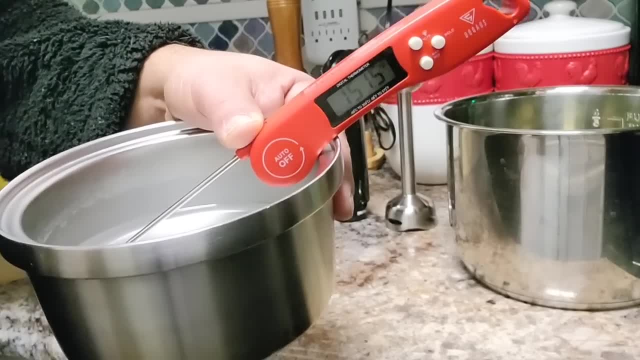 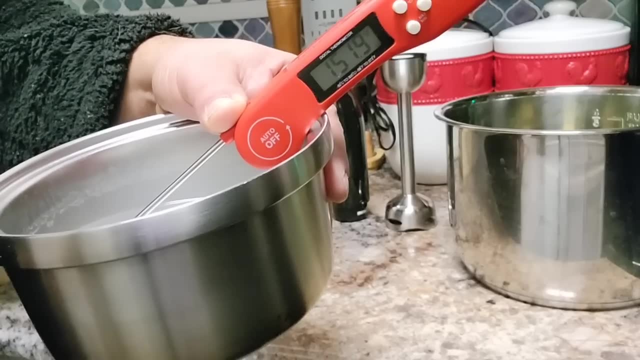 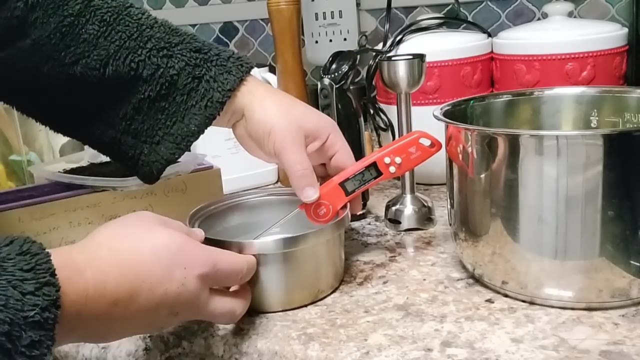 but that says: what about 152 degrees? So I left this outside in the cold for about 15 minutes or so and it's still about 150, 151 degrees. So we have to let this get down to below 130.. Once it gets below 130, we are then able to add about a half a tablespoon of our sodium lactate. 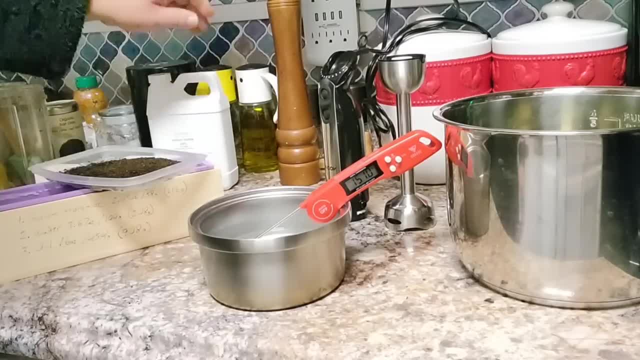 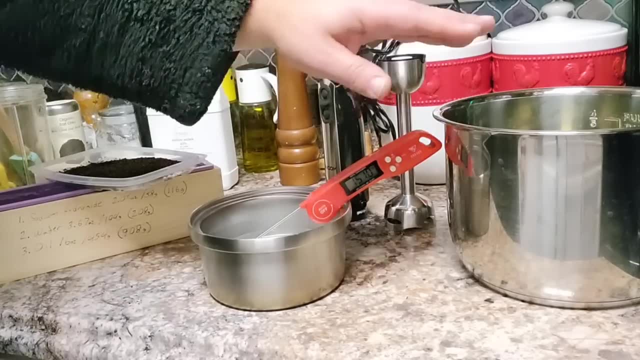 right into this water before we mix it in with the oil. Once it gets below 110 degrees, then we're going to go ahead and mix it in with the oil Once we preheat our oil to about 100 degrees Fahrenheit that is. So let's give it a little bit of time so that it can do what it has. 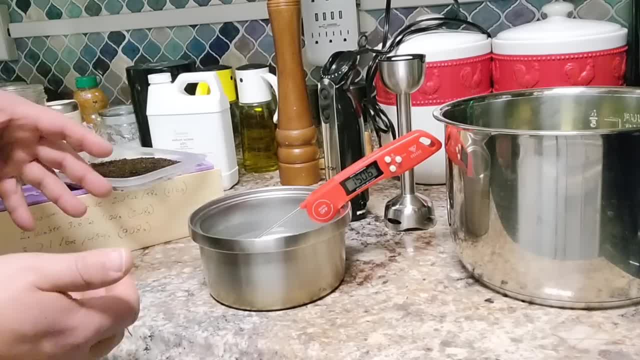 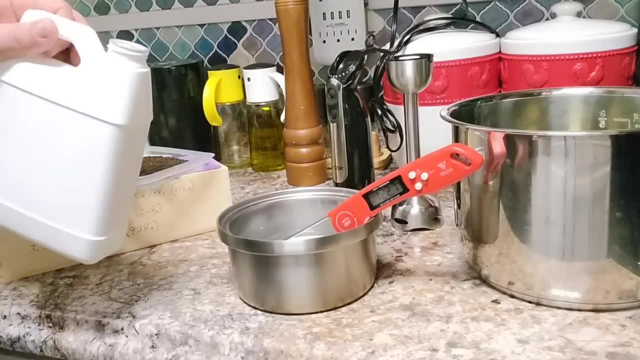 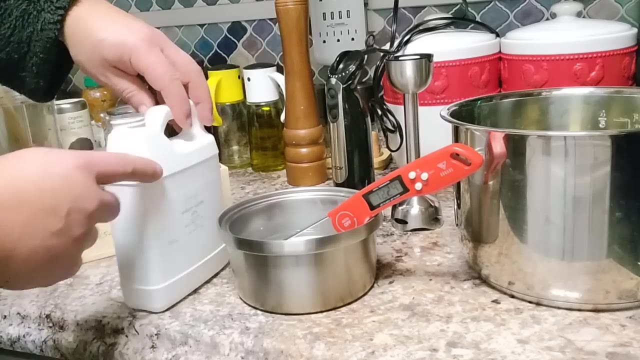 to do, naturally, instead of me trying to rush the process of cooling it down. All right, ladies and gentlemen, the temperature is at 123, or just shy of 123. So we're going to add. Now, this is a double batch, so it calls for a full teaspoon of this right here. the sodium: what is it, Sodium? 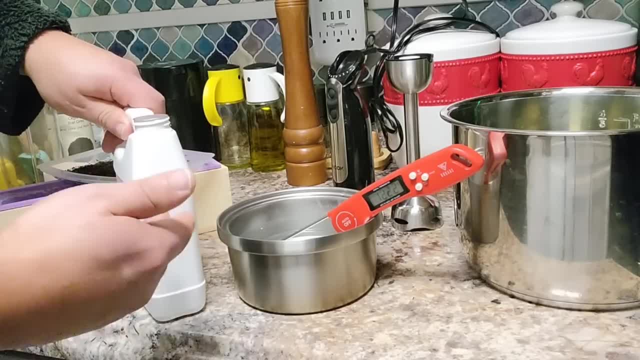 lactate. But I've found that using like a half of a teaspoon is just fine, So I'm just going to dribble it in And then I'm going to add a little bit of water, And then I'm going to add a little. 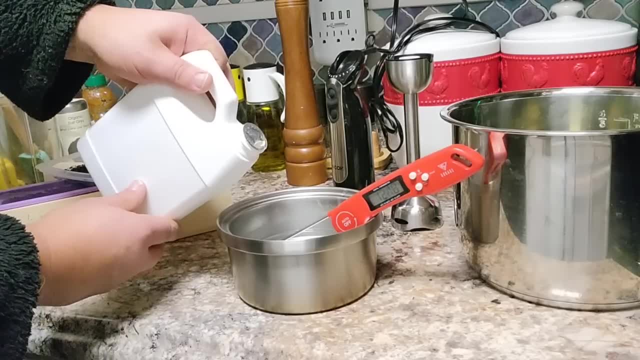 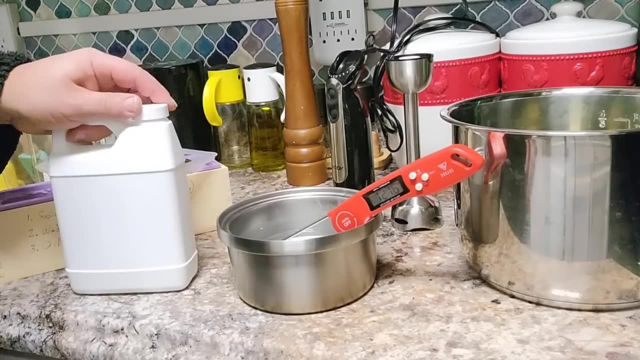 bit on there. I'm not going to measure it. It's no big deal Right there. That right there is going to be just fine, And that way you don't have to be waiting all day long for your soap to harden up. 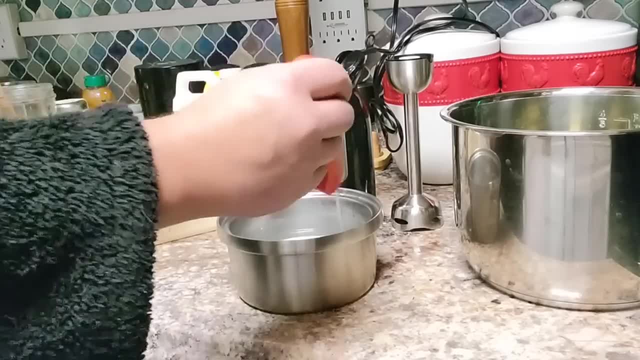 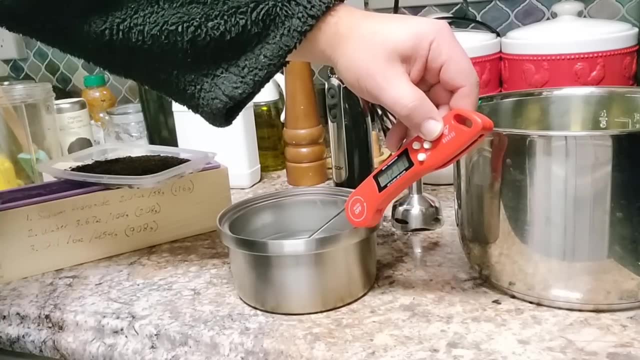 We're just going to mix that around there a little bit. Our temperature is down to about 121. Let's see Yep 121.. So now I'm going to bring the temperature of the oil up to about 100,, 110, and then we'll be out there, And then we're going to bring the temperature of the oil up to. 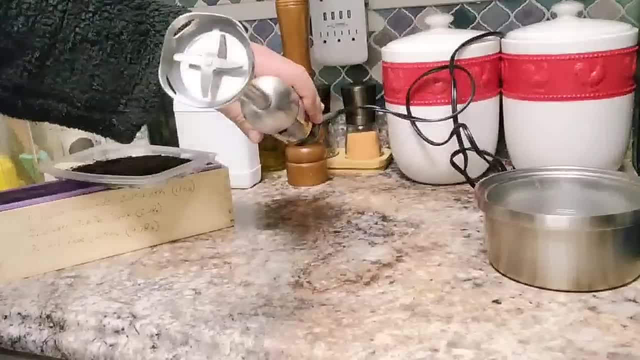 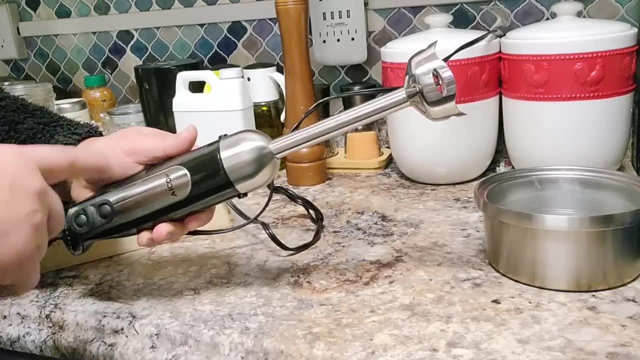 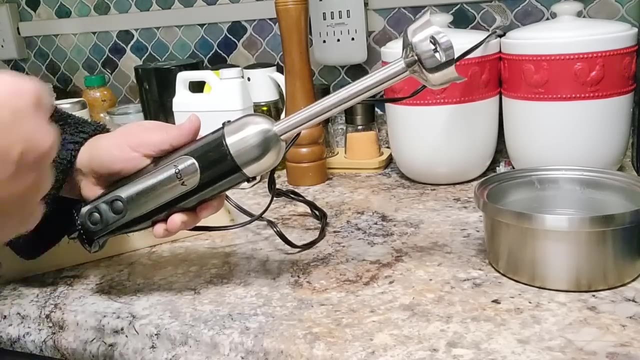 about 100,, 110, and then we'll be able to mix these together Now while our oil is heating up. ladies and gentlemen, I did fail to mention that you don't have to have an immersion blender to do this, but it really is nice to have one If you have plenty of time and you don't mind stirring. 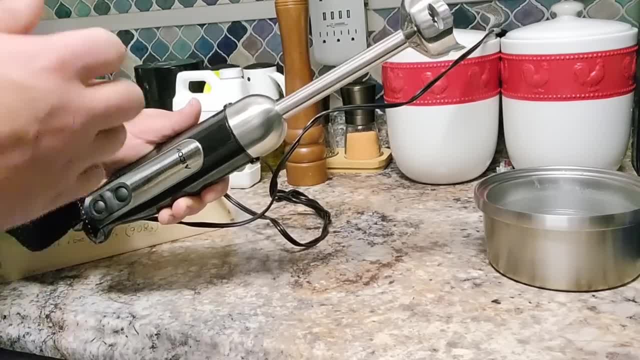 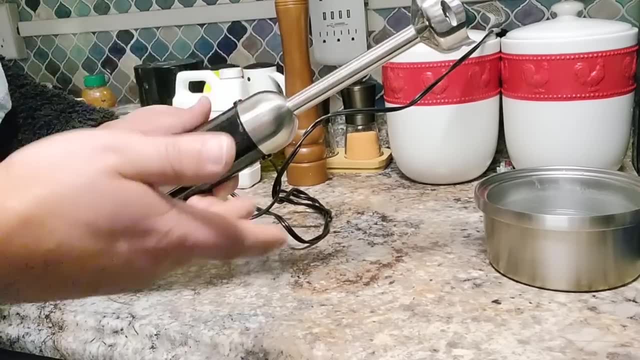 with a wooden spoon or a stainless steel spoon for a while, then that's fine. You can do it that way, But this makes it so much easier. You'll be done getting your trays in about two minutes, maybe three or so. So an immersion blender is a great way to do this. So I'm going to bring the temperature. 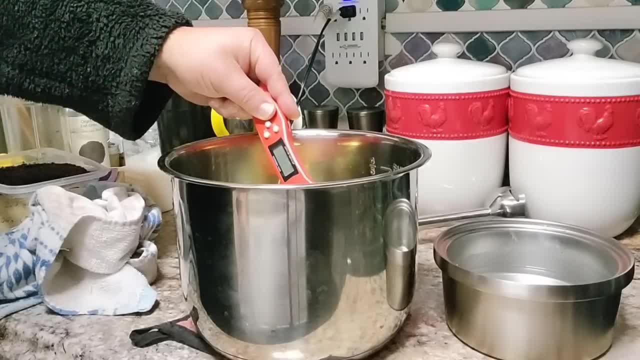 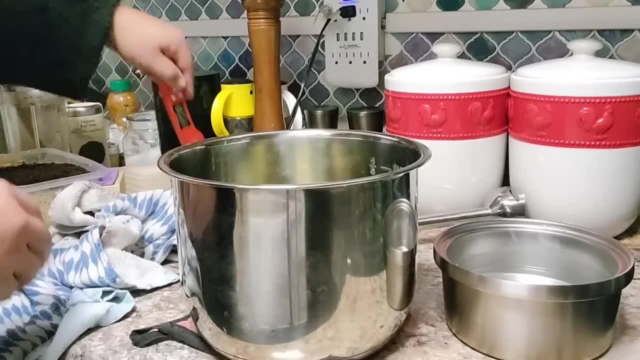 up to about 120 degrees. So an immersion blender really does help. Let's see 103 degrees, right, 102.9.. That is good enough. Now we're going to go ahead and get our water Again, ladies and. 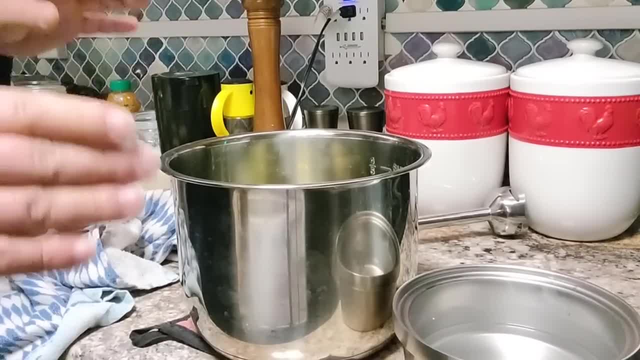 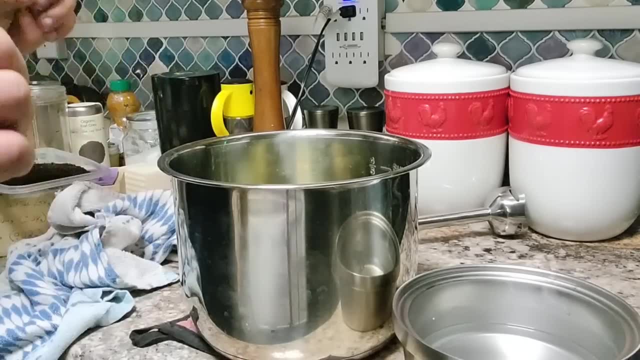 gentlemen, I stress that when you're doing this, use personal protective equipment, ie glasses and gloves. You don't see me using gloves here, but it's not because I'm not advocating that you do so. All right, make sure that you use gloves and make sure that you use. 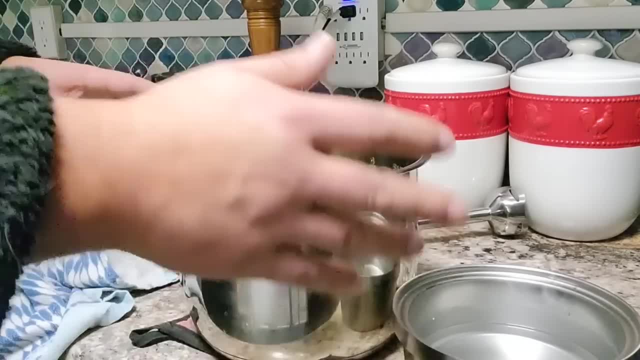 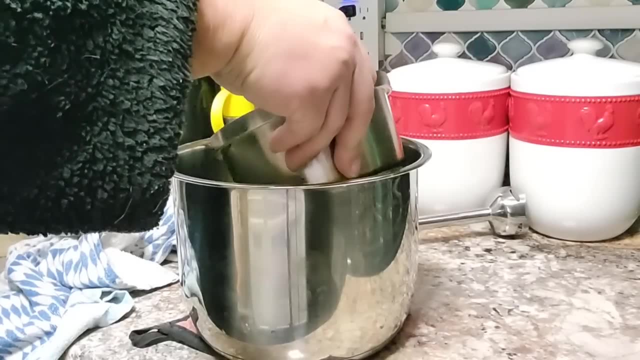 something for your eyes, just in case you get a splash. This is not going to create any kind of boil over or anything like that. It's going to be just fine. Just be very careful when you're putting it in. You don't have to be in a rush. I'm going to put that in there And as soon as I put. 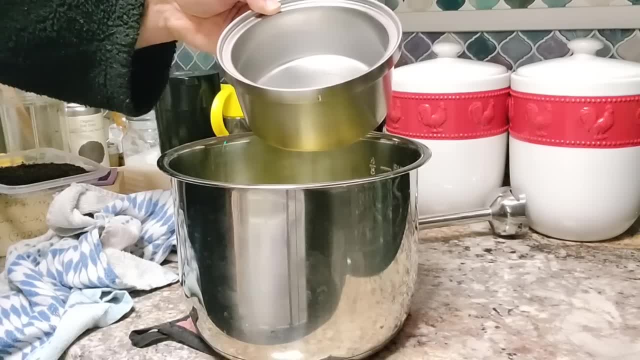 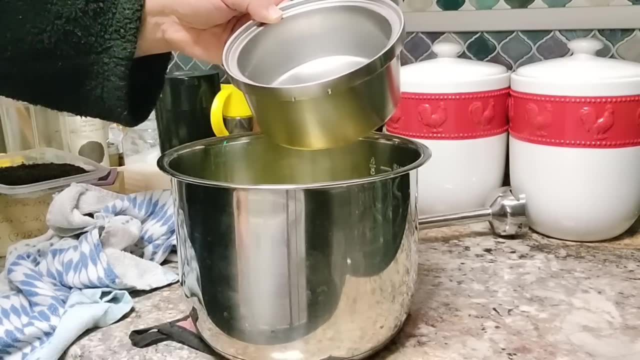 that in there. I'm going to go ahead and put this in the sink and fill it up with water. Why? Because dilution is the solution. You don't want to forget that you put this in your sink and then someone go in there and touch it with their bare hands and get burnt. All right, this is the. 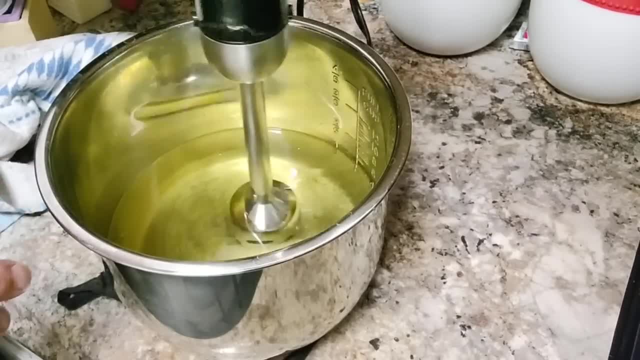 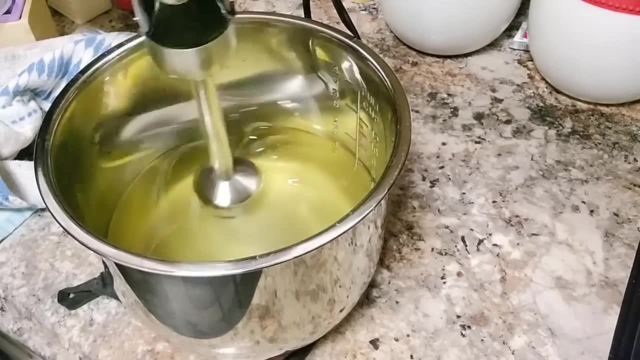 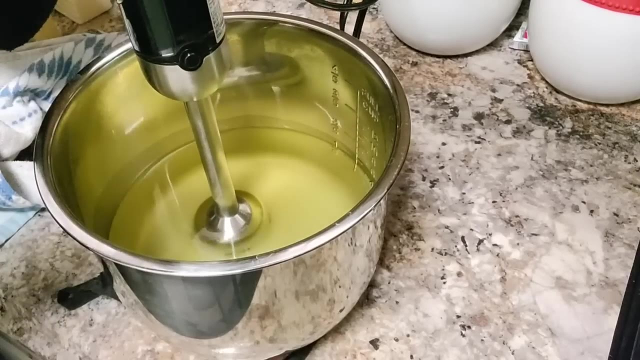 best that I can do as far as the camera angle. right, This is not Hollywood here, ladies and gentlemen. So now that we've stirred it around and we've kind of like spread it throughout the oil mixture, now we're going to go ahead. I'm going to put it on a low setting and I'm just 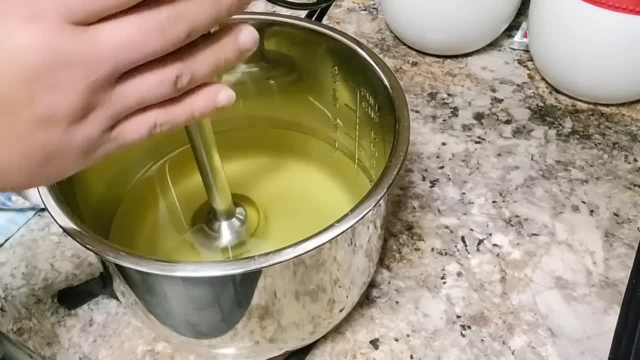 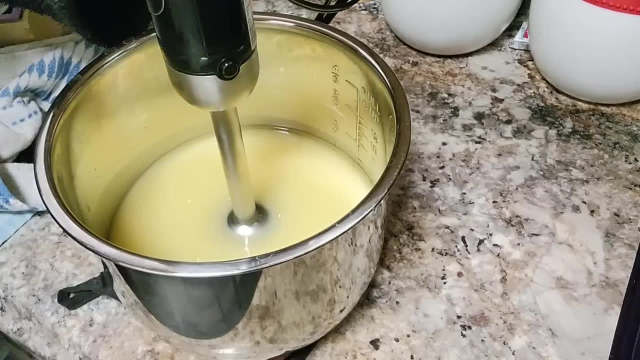 going to pulse it. All right, I'm not going to put it on all the way, I'm just going to pulse it. Now, ladies and gentlemen, all I'm going to do is I'm going to continue to do this until we find. 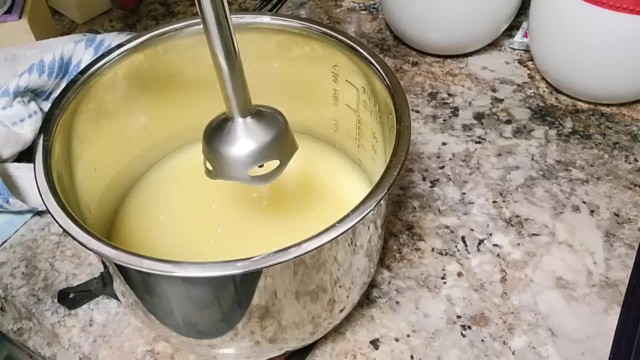 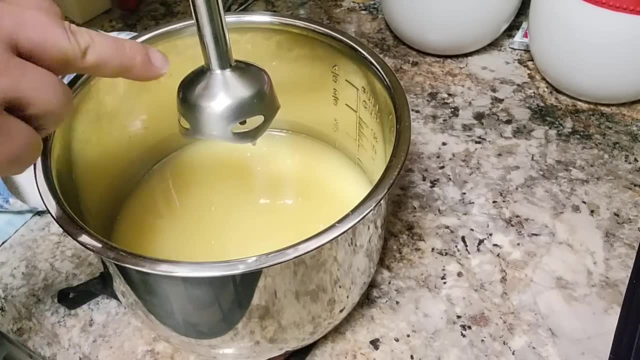 trace, Like right now. you can see there's no trace Trace. the way that I identify trace- and there's different ways of doing it- is if you can go ahead and put your finger down and you can see that the soap stays on either side- It doesn't fill in- Or whenever you can drop, drops into the. 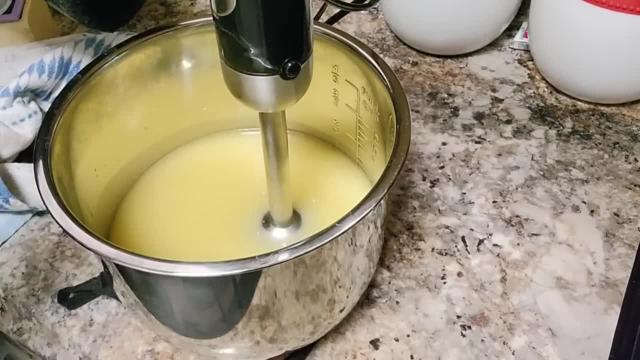 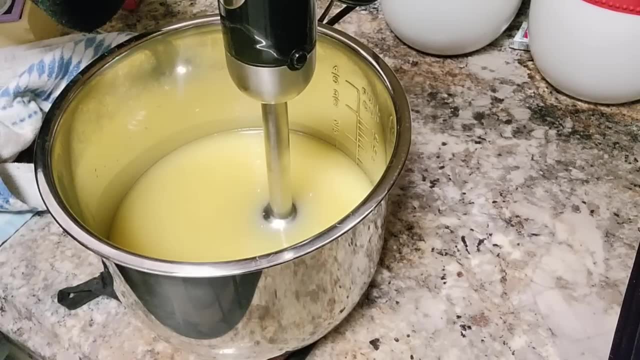 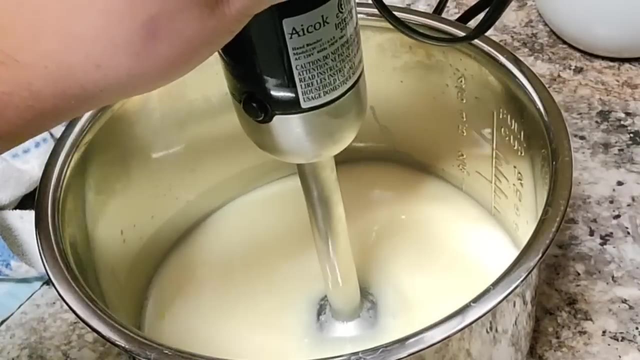 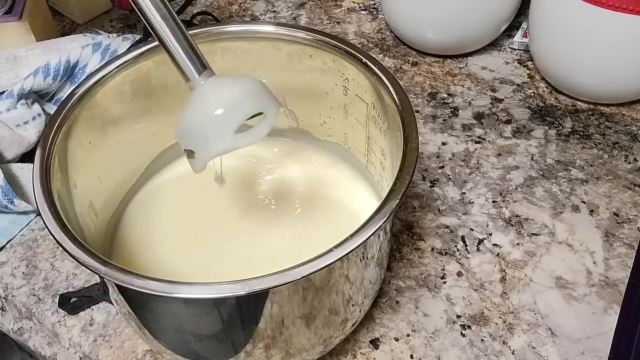 mixture and you can see that it makes a dimple that stays there for a while. That's what I consider trace being. I'm going to continue to do this until I find trace, And then we'll go to our next and second to last step. Now, there you go, ladies and gentlemen. That is what I call trace, Some. 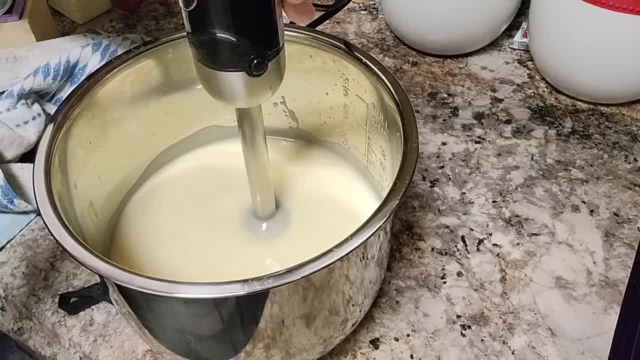 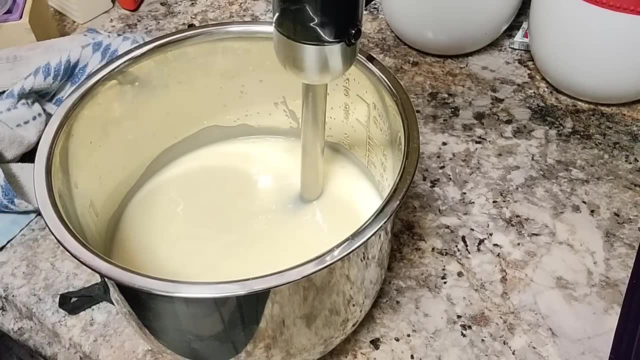 people may want it a little thicker, but the truth is is that even if it wasn't this thick and it was thinner, it will still set in your mold. It'll just take a little longer. So now we're going to go ahead and add our vanilla and tea mixture. 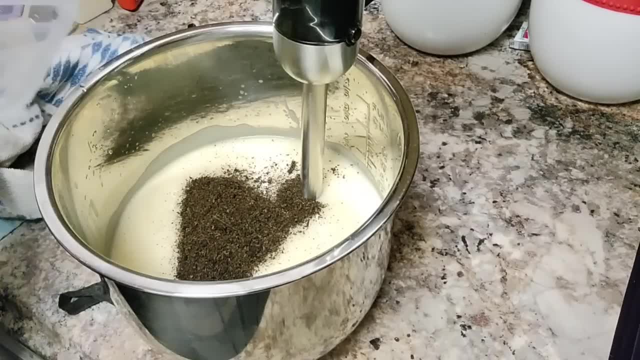 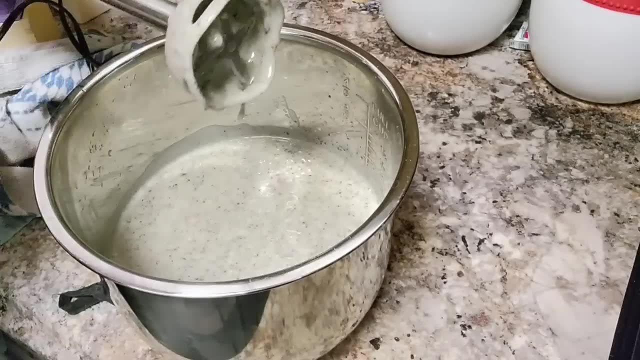 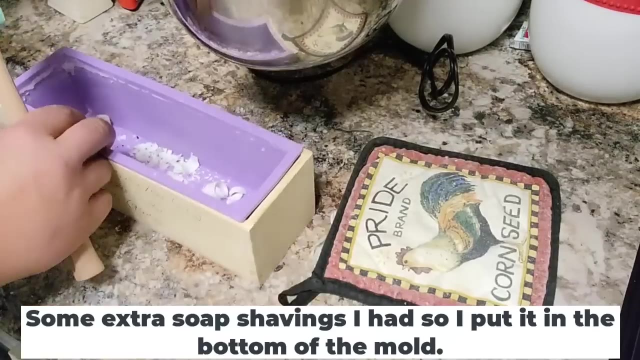 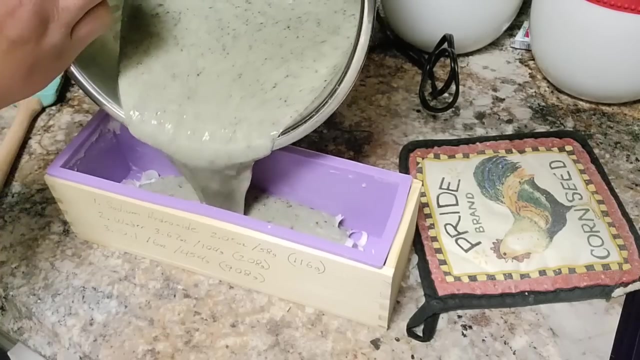 And this smells really good. Let me tell you that That vanilla and tea, And we are now ready to pour this into our mold. Now we're going to go ahead and pour our mixture into our mold, And this should be just enough to get our mold pretty much full to the top. 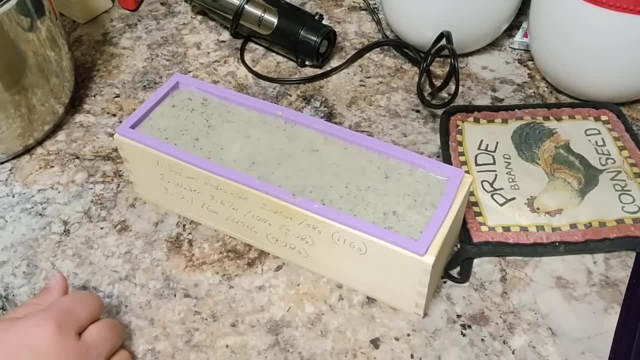 And there you go. Now we're just going to let this sit here, probably for about two or three hours, And then we'll come back, take it out of the mold and show you how easy it is to cut up One thing that you don't. 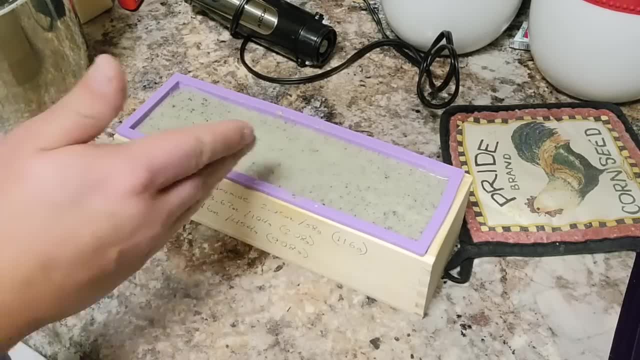 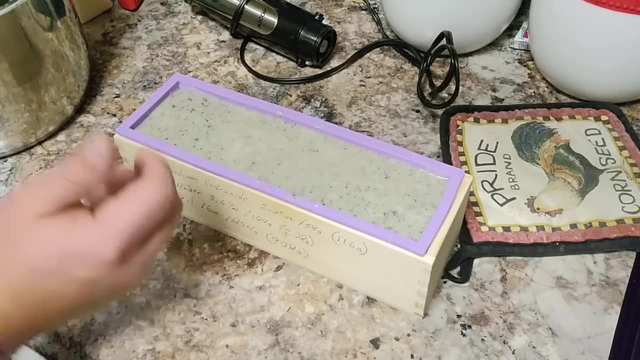 want to do, though, is: you don't want to let this sit here for a couple of days in a mold like this, because you're going to want to cut this, And the longer it sits, the harder it's going to get, and the harder it'll be for you to cut it, And after about five or six hours, 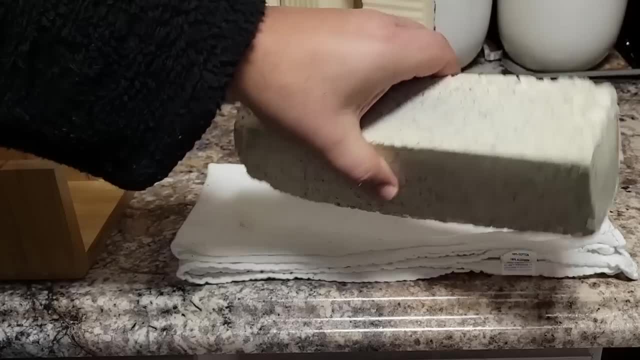 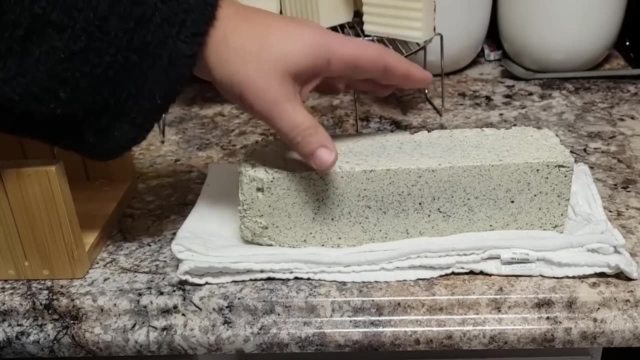 ladies and gentlemen, this is what it looks like- Like a big block of speckled cream cheese, I guess you can call it. And the reason I didn't show you all me taking it out of the mold is because I'm a one man crew and it's kind of like a pain in the butt to take it out of that mold. 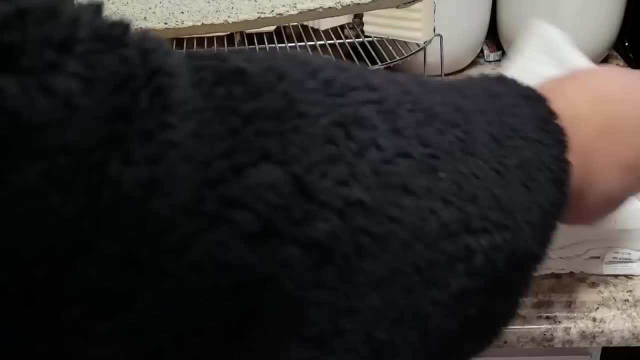 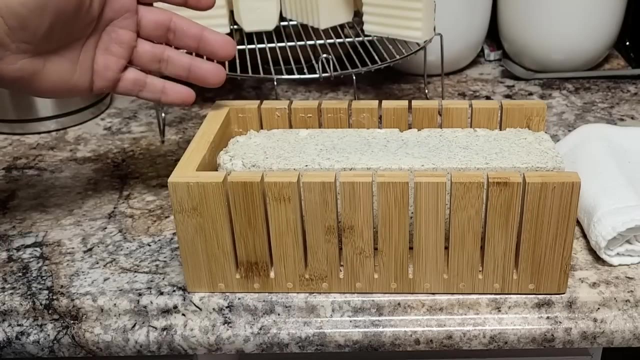 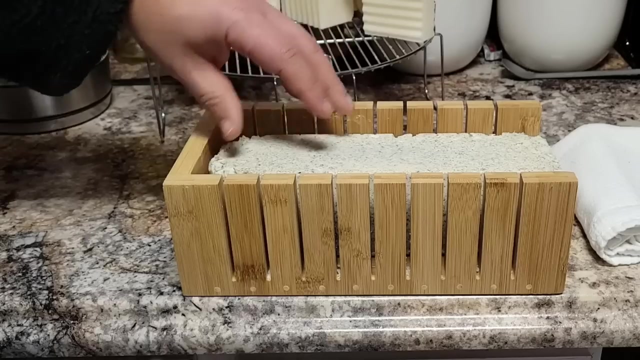 So I went ahead and took it off without the camera on. but pretty simple. Now, all we do is, if you go ahead and buy, there's a small kit that you can buy like a soap making kit, And it comes with something like this: You don't have to have this, but it is kind of handy when. 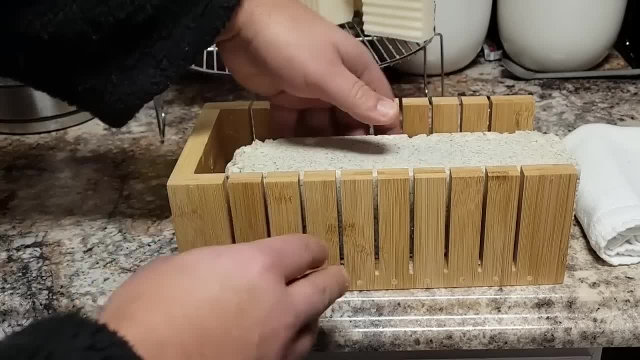 it comes to cutting up your soap into even pieces. So I'm going to go ahead and show you how it looks. You're going to need even pieces, I guess you can say, And what I like to do is: I like to take the 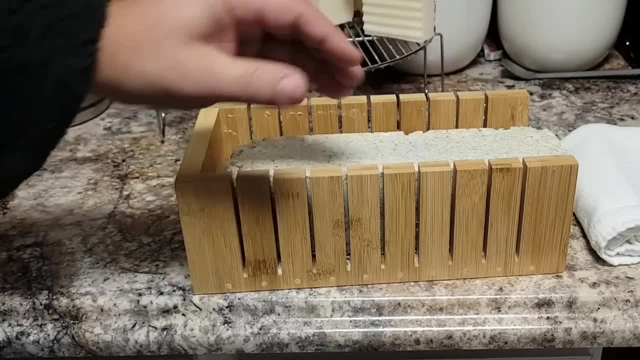 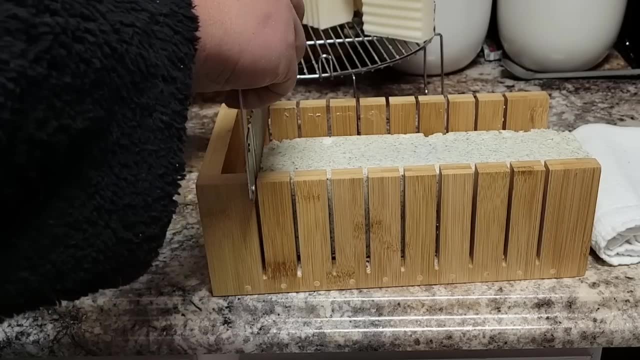 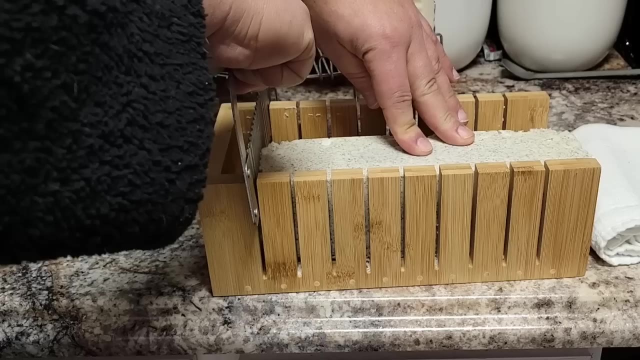 edge off and then cut them in pieces that are a little bit thicker than normal. Let me just show you. So here is our first cut, And it's good to do this now. You don't want to wait like days before you do this, because if not, your soap is going to be really hard and it might break when. 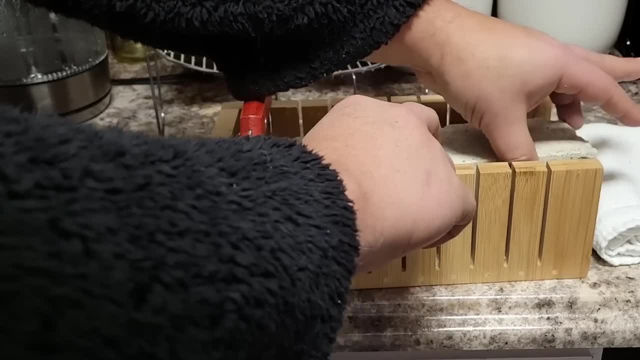 you do this, But, as you can see right here, I just cut it in half And then I'm going to cut it in a small piece off the end And you can see right here that this is the piece that's kind of ugly. 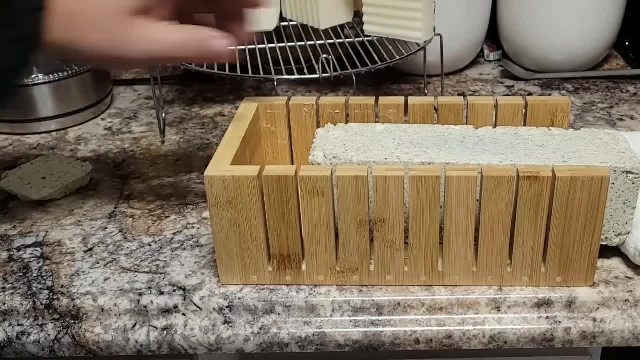 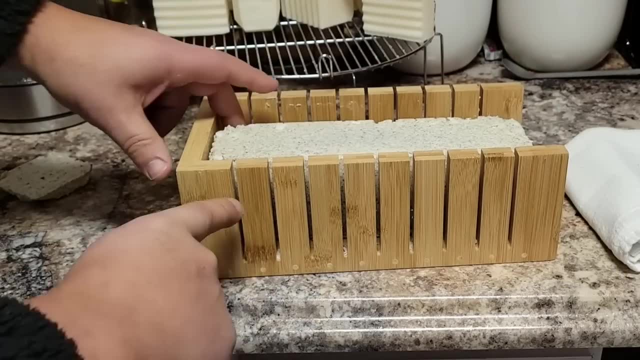 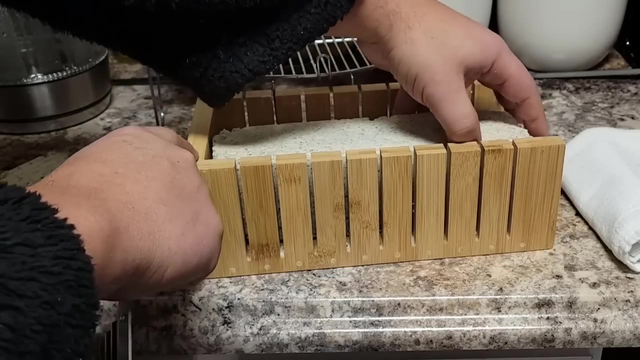 right, But this is still soap, so you don't get rid of this, right? You're going to keep this, And I like to cut these in a little bit thicker pieces. So, if you take a look, we have like one inch pieces that you can cut them in, but I like to cut them in pieces that are about an inch and 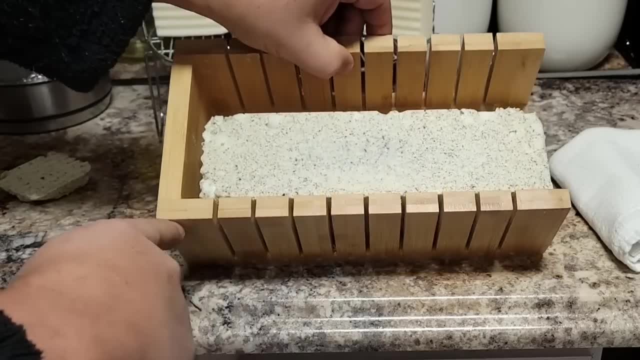 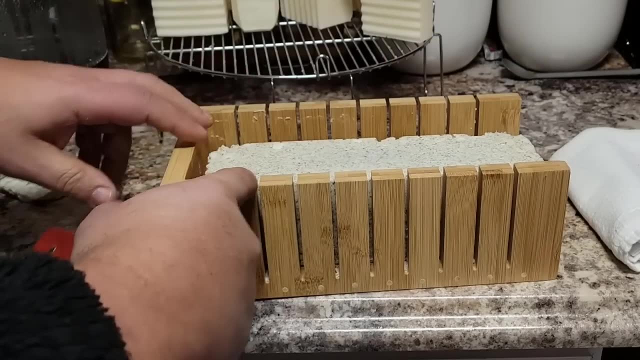 a half. So I'm just going to go ahead and bring this About halfway to the mark right here, And then, instead of cutting it here, I'm going to cut it there. Check this out, Let's see if you can see this. All right, So we're going to line this up. 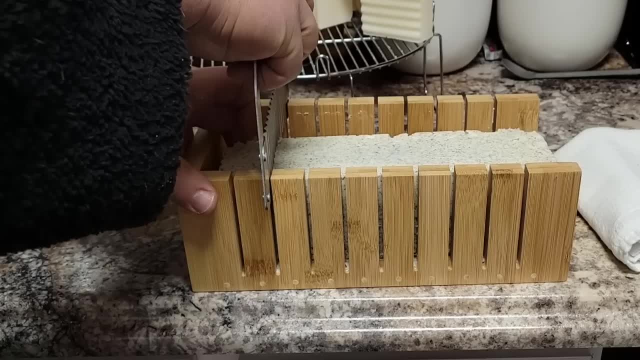 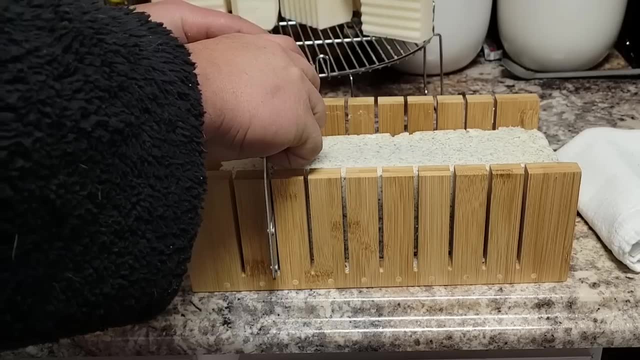 And we're just going to go right through: Nice and easy, And it is still nice and soft. And, like I said, if you do this now, it'll be nice and soft and you won't break the soap. But look at. 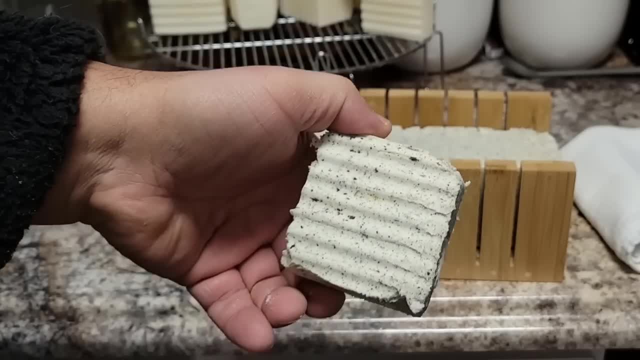 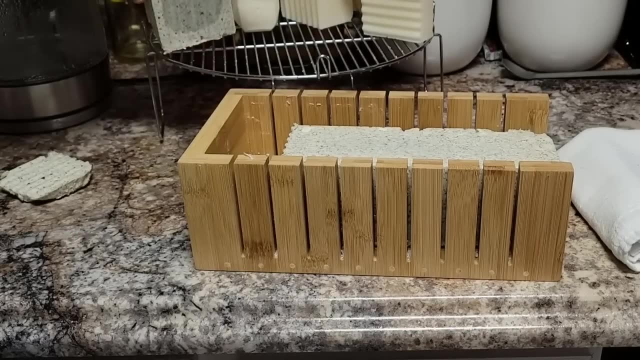 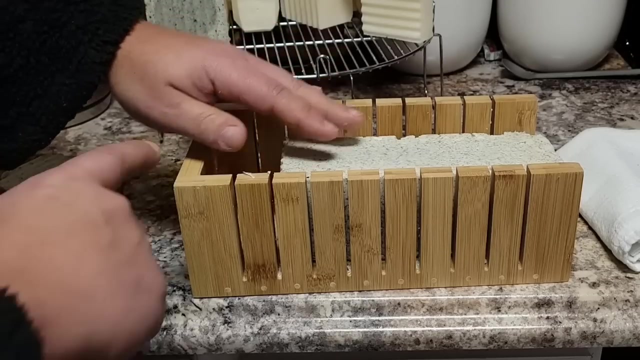 oh, look at that. Look how pretty that is in the middle. like that You can see the middle there hasn't really cured yet. This is actually curing still. It's almost like concrete, right? This actually gets warm When you put it in here. it stays warm for a long time because it's still 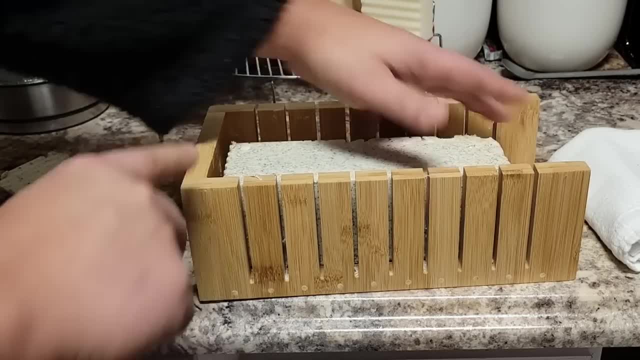 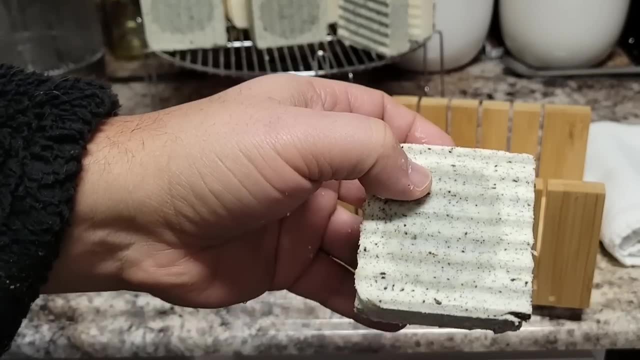 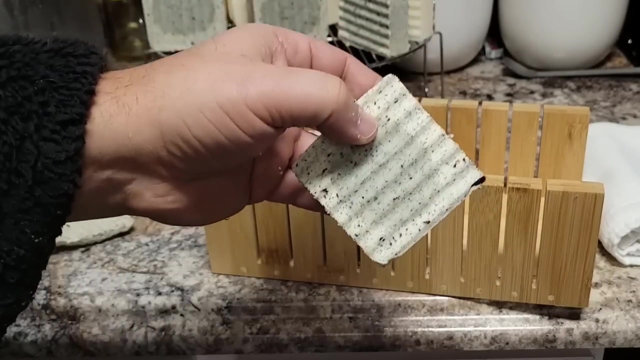 curing. So I'm just going to go ahead and keep doing the same thing. I'm going to keep doing a, about one and a half, And then you can see that these are pretty nice And they actually smell halfway decent. They're going to smell a lot better, actually, after they're. 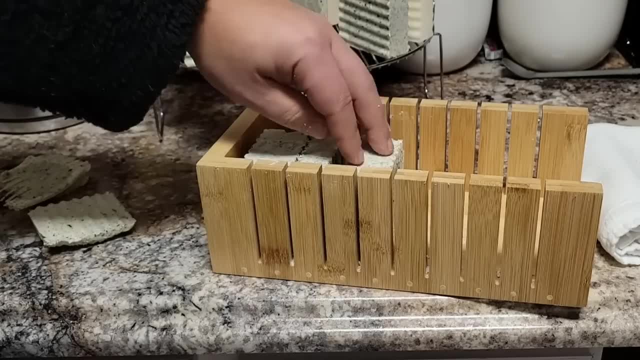 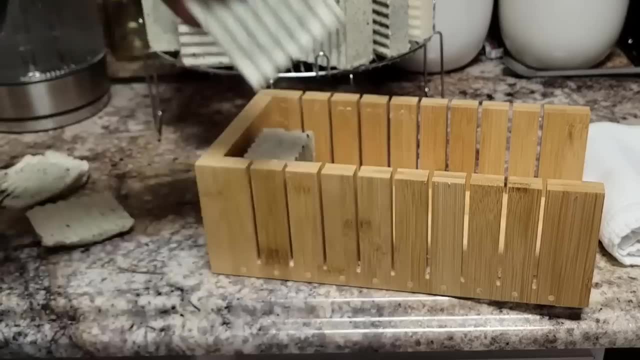 completely cured. after they're completely dry, You can see that these are still wet, So normally you would probably want to leave these on the rack. that you see me putting them on here probably for about four or five weeks really is how long I leave. 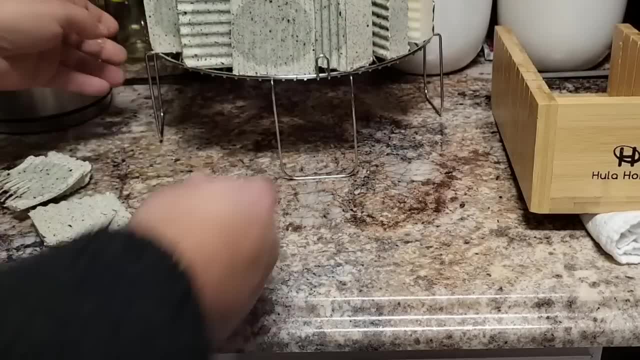 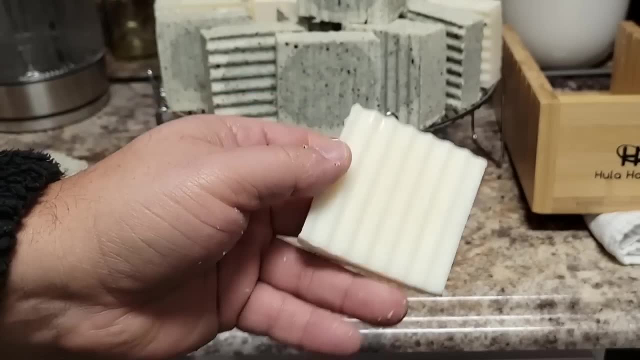 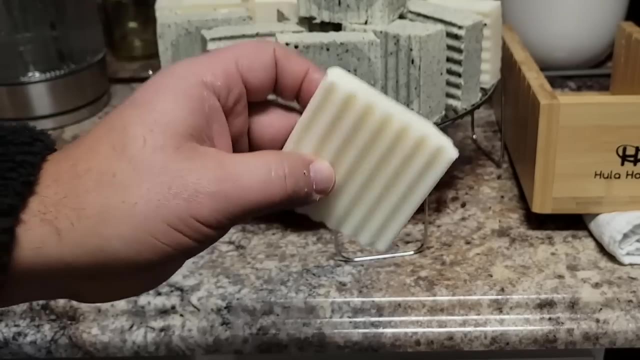 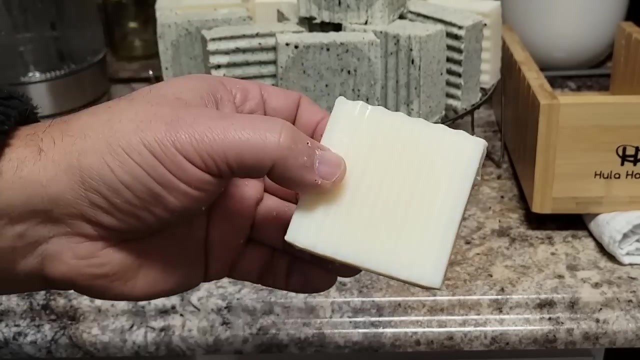 But they can come off a little earlier, Like, for example, this one here is only about a week and a half old or so. This is the one where I made it with a pure olive oil or extra virgin olive oil with some coconut oil, And this is about almost 10 days old or so And it already starts to